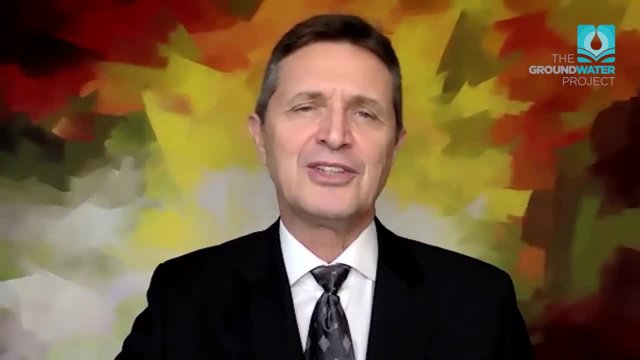 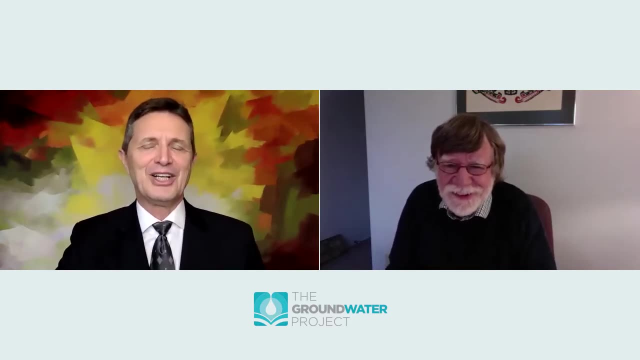 geothermal systems and contaminant transport in heterogeneous porous media and fractured bedrock systems. Well, a lot of things, Very good. You will get a lot of information because of the work that you do, Thank you. Les is a very experienced guy. He's seasoned in mining information. You'll love it. 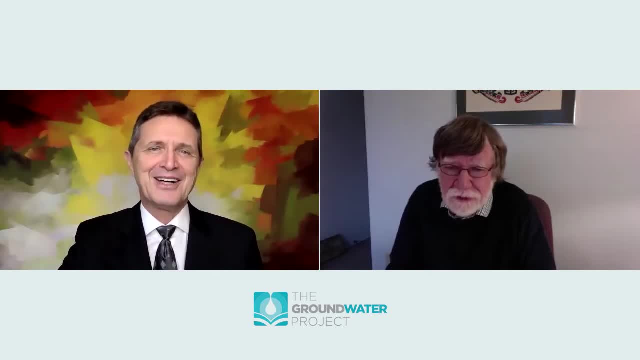 Okay, Les, thank you very much for participating in our Groundwater Project. It's an honor having you here, Please. your book presents a very good view of hydrogeology in the mining industry, which reflects your career, of course. Please tell us a little bit about your career. 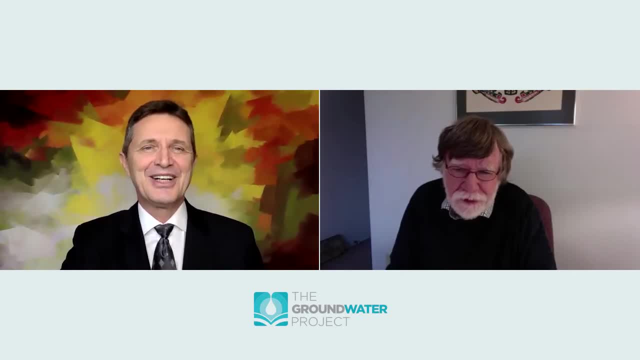 For someone who doesn't know you what you've been doing, know how you arrived to the mining industry and how you've been a success there. Okay, I have an undergraduate degree in geology from the University of Alberta, where my first 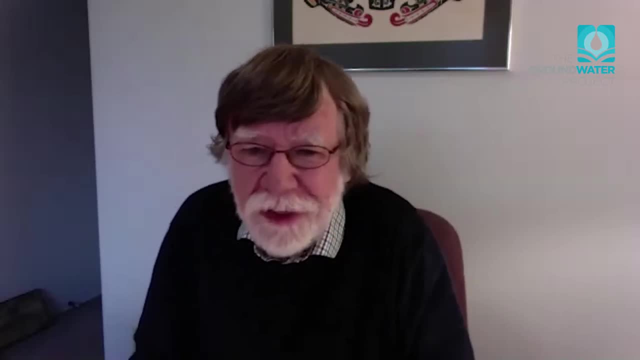 course in hydrogeology was with Frank Schwartz, And then in mid-70s I went to the University of British Columbia where I did my PhD with Al Fries. After that I went to University of Utah for several years and then came back to Canada and spent the bulk of my university career- I think 35 years. I was a 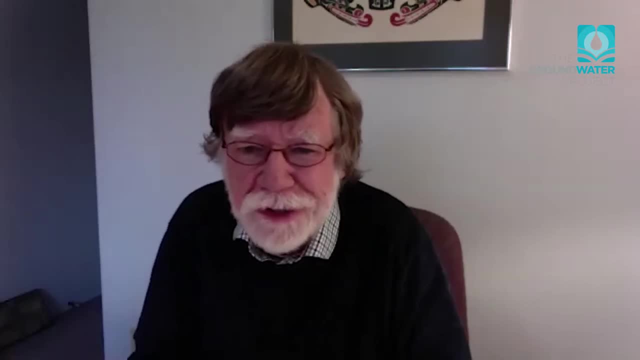 professor in the Department of Earth, Ocean and Atmospheric Sciences at UBC, I retired from there about five years ago, And since that time I've been working as an independent consultant on technical review boards for mining companies both in Canada and internationally. 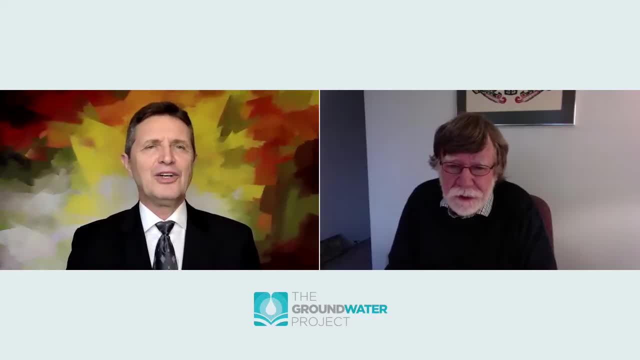 Oh, very good, Very good. Well, your book starts with climate and geologic settings. How important is climate? Well, we're talking a lot about climate in this day, right? How important is climate, for that matter, for hydrogeology and mining industry? 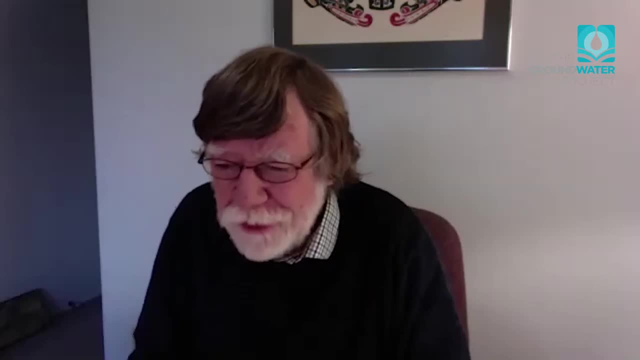 Climate's key, because one of the general rules in mining is that water is almost as important as the ore that they're mining. So water availability, management of water, is a key part of the activities on the mining industry, And so I think for me it's a key part of the activities on the mining. 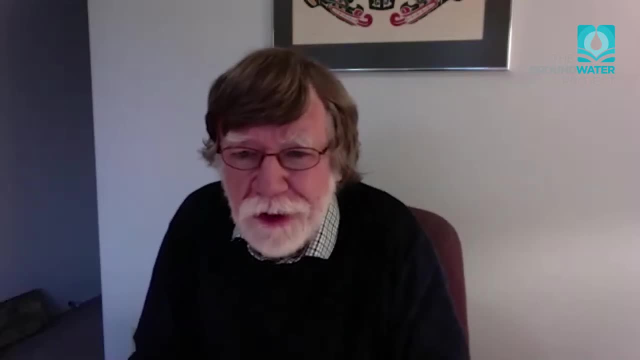 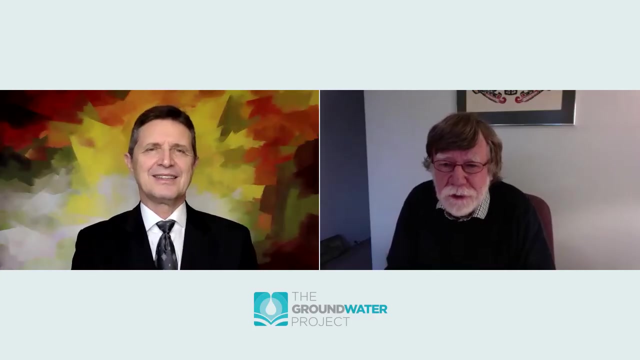 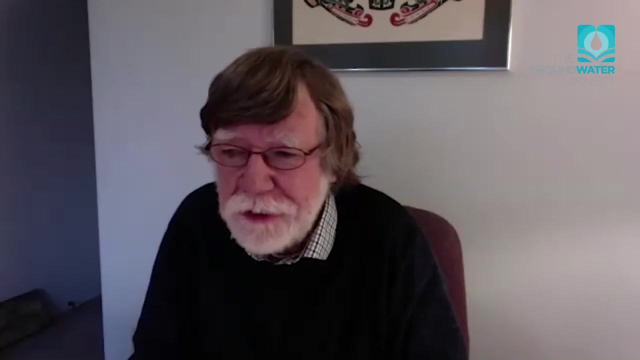 industry, And so I think, for me it's a key part of the activities on the mining industry And so, essentially, the broadest range of climate we have on the planet is what the mining companies need to operate in or operate in, And that determines temperature And that determines the quality of the. 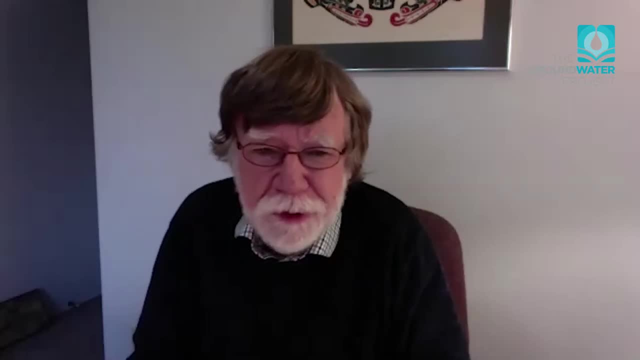 temperatures, precipitation, seasonal distribution of precipitation determines the amount of evaporation. All of those factors go into determining groundwater recharge And, as you know, groundwater recharge determines depth of water tables, which has implications of if you're excavating below the water table, you're going to have fluid inflows. It determines water balance. 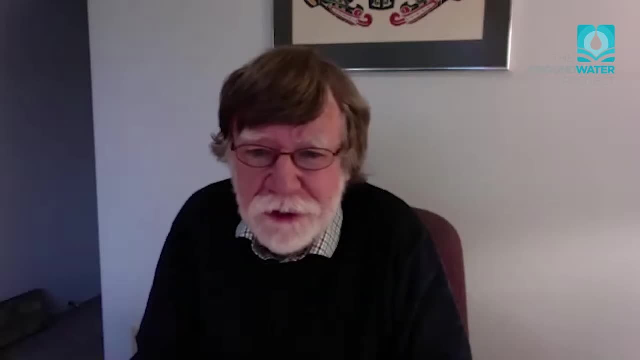 whether you have an excess of water to manage at your site or you have a deficit of water. In other words, evaporation is greater than precipitation. If you have a deficit of water, then you have to find the water from elsewhere, Either surface water or many mining companies. 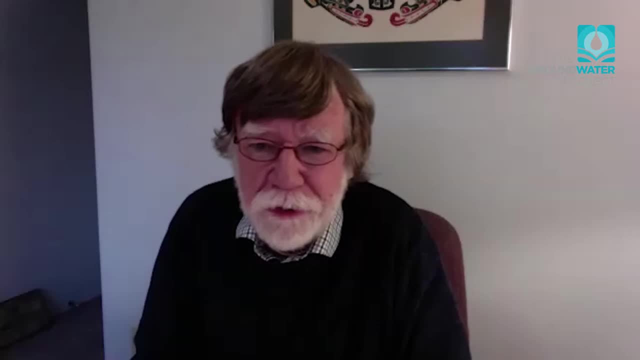 use groundwater resources to provide a supply of water to their processing facilities. So climate sets water availability and the general framework- general hydrologic framework- in which they occur. If you're in the Canadian Arctic, the groundwater problem is set by the permafrost distribution, for example. Another example of how the climate 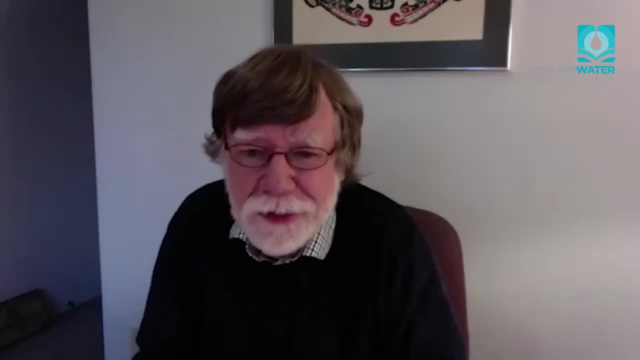 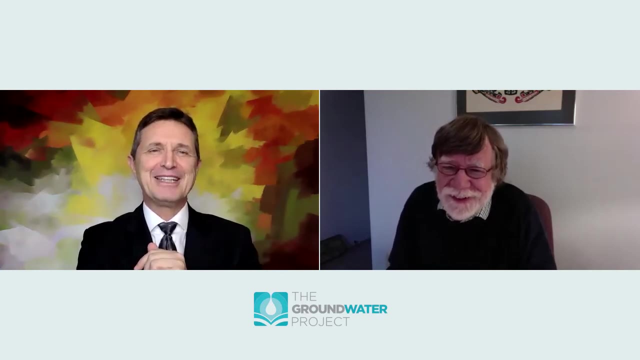 determines what the hydrologic system is at a mine site. Okay, For someone who doesn't know exactly, for someone who's from Brazil who have a very great idea of what a permafrost is, could you explain better that for us please? Okay, In Northern Canada there is a zone called continuous permafrost. at one of the lakes where I've worked there, The water- if you like the groundwater- is frozen down to a depth of 250, 300 meters. So the recharge systems there occur from lake to lake to lake. because there's an unfrozen zone beneath the lake, Then between the lakes, the groundwater doesn't move because it's held up, bound up in ice, So it has a major impact on the character of flow systems in comparison to a normal system we'd experience 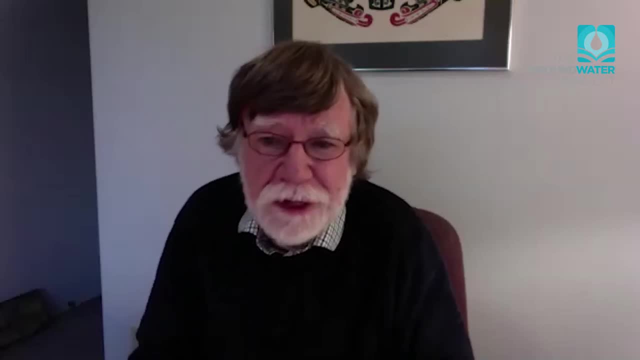 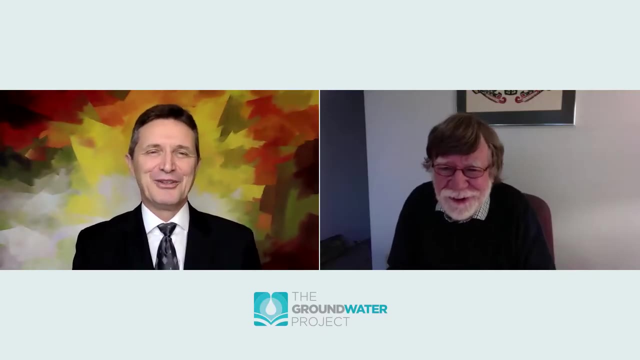 A system that we'd normally encounter in sort of the Canadian prairies or the US Midwest, Yes, Where topography controls the flow. You know, because I first saw real snow, for sure, you know, in Canada, When I was, you know, after my graduation. you know that was after my master's. 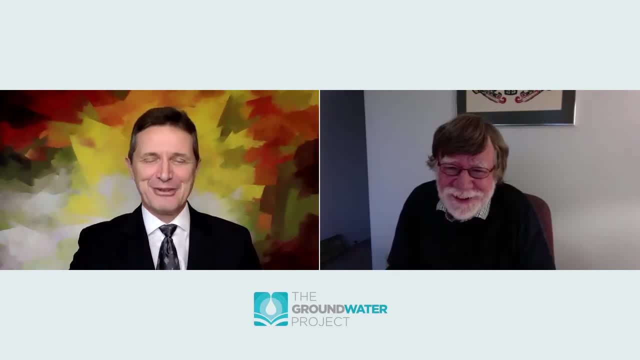 Yeah, That's typical. for a Brazilian and for lots of people living, you know, the equator down, That's very typical. Well, my related story to that- this is a side comment- is we have a dog from Mexico and it was six years old when it came here And, of course, it had its first snow experience. 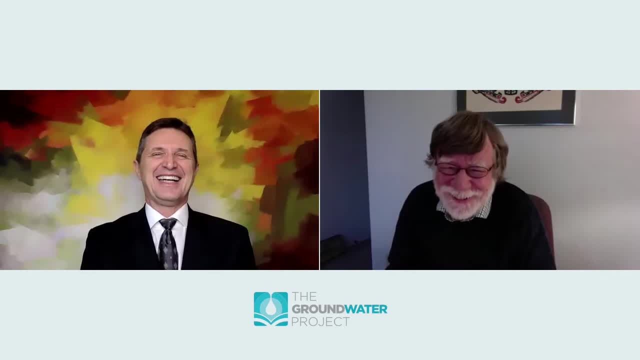 and it's a husky Wow. I can understand how you probably have felt when you first saw snow. Our dog didn't know what to do with it. Exactly, Exactly Well, but I got used to it. I lived for five years in Canada, so I got used to it. 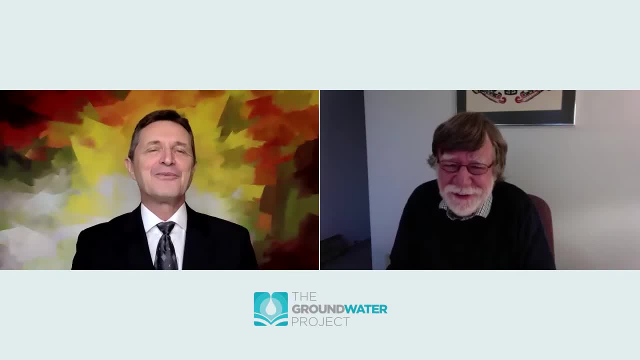 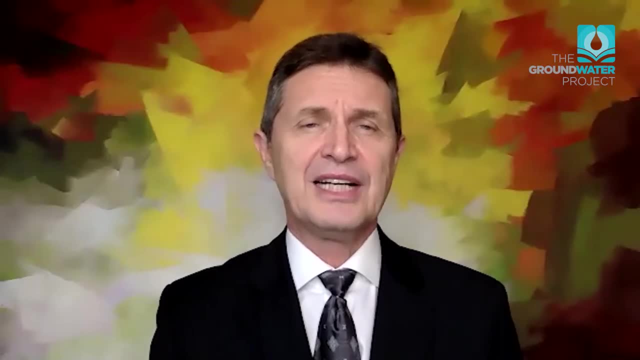 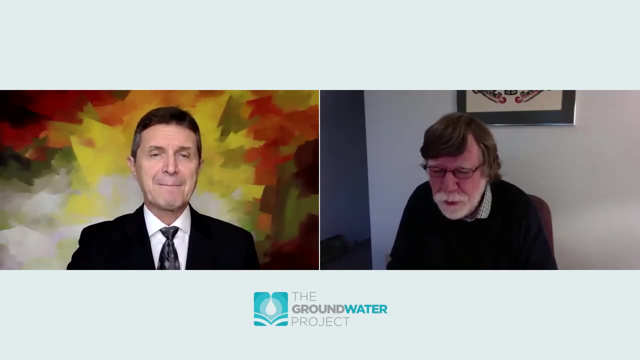 I know the problems and I know the beauty. Yeah, Again, you're talking about the climate, but what about the geologic setting as well? Because it's also related to hydrogeology, right? Can you tell us Exactly? So, just like climate has a very broad range. 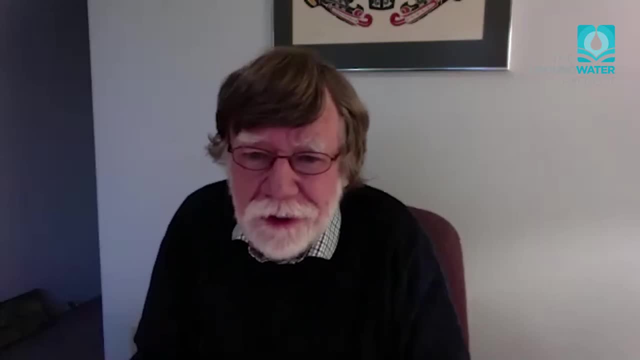 mines occur in a very broad range of geologic settings. They can occur in shield areas, as in Brazil, or in Canada or Africa. They can occur in sedimentary basins, so you can deal with igneous rock, metamorphic rock, sedimentary rock In the Andes. everything is a combination. 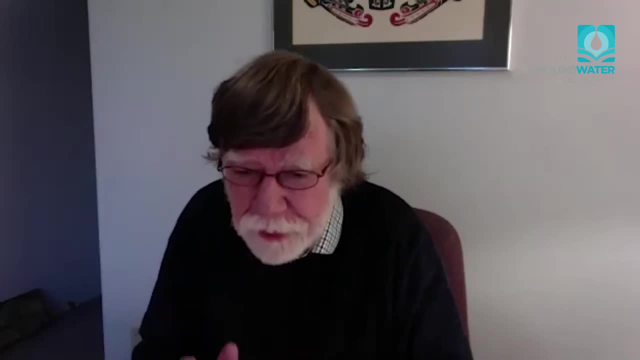 in the sense that you have the igneous bodies coming out forming the ore deposit, but they intrude through thick limestone beds. so you're dealing with issues of karst, for example, And my experience is that when operations don't go according to plan, 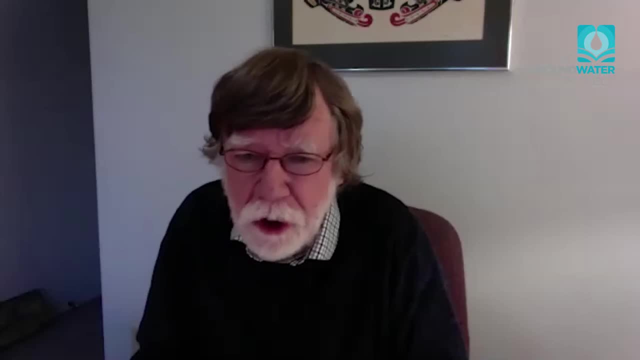 it is often the case that there was some feature in the geology that wasn't anticipated ahead of time, so you have excess water inflows. So really to understand the water inflow potential along fault zones, for example through karst features, you really need to understand the 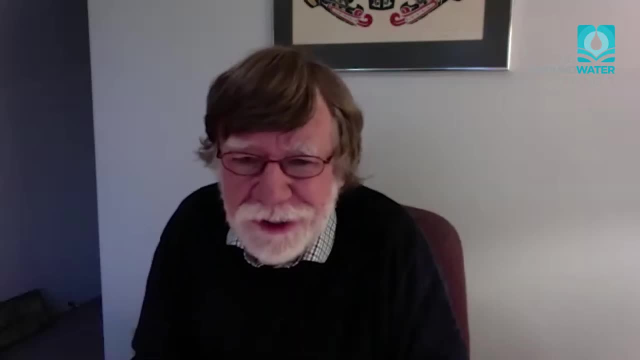 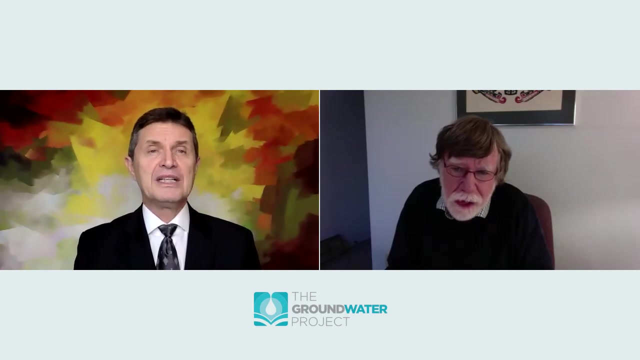 geology as well. You can't do hydrogeology on mining projects without understanding both the water and the rock And interaction between both right And the interactions between them. Very good, very good. So when advising an investigation for a mining development, 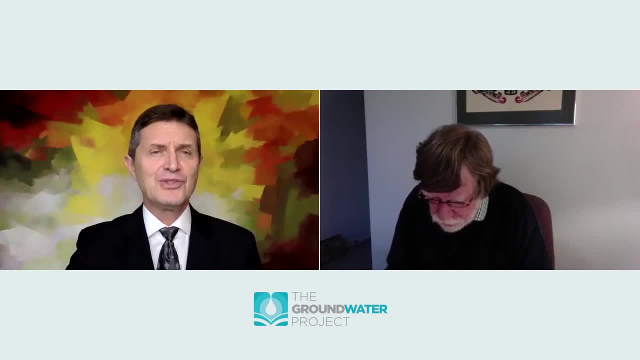 how is hydrogeology important and how is it used for that? When you're doing a site investigation, you have to think about, for example, if it's an open pit mine. you have to anticipate how much water may be flowing into the open pit mine as it's being developed, as it goes deeper and deeper below the water table. 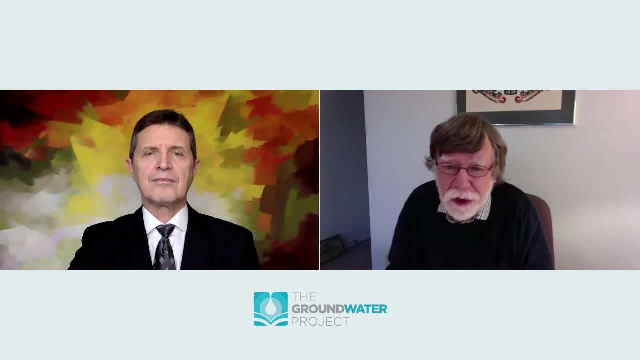 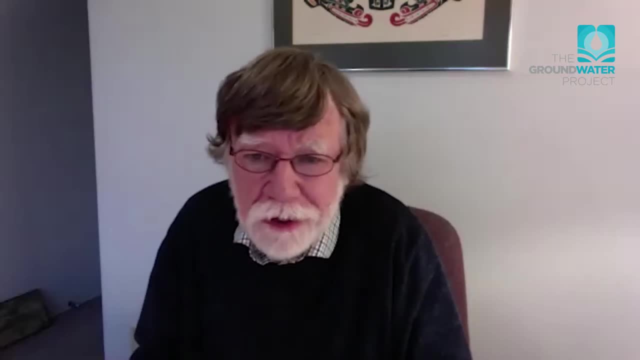 And so you need to characterize the hydrogeology in the area of the open pit or in the underground workings. If you have a high permeability bedrock in the area, for example, and you have high rainfall, you can anticipate larger inflows, So you have to have a means of managing that. 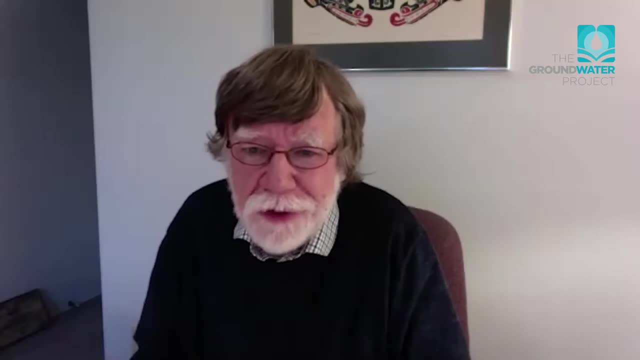 what volume of waters need to be managed, And so for that you have to have a site investigation program. For a tailings facility, there are foundation conditions. the strength of the foundation depends upon pore pressures in the bedrock, And so you need to have a 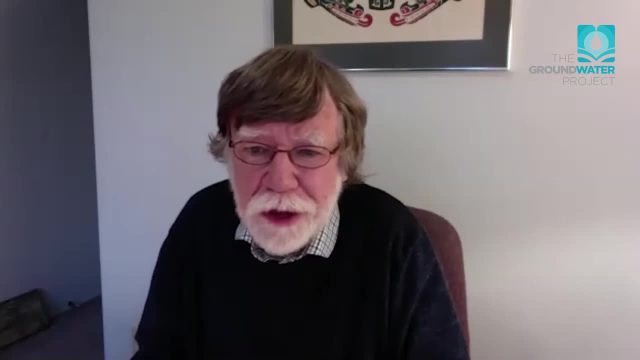 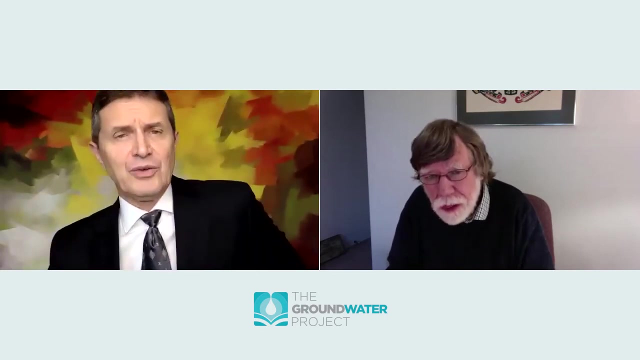 characterization program to find the most suitable location for a tailings facility, So that is safe and doesn't require a lot of mitigation measures to make it safe. I think that, yeah, that's it for that. I think Right, right, So, but then, well, let's say, okay, we go there, we have a very good 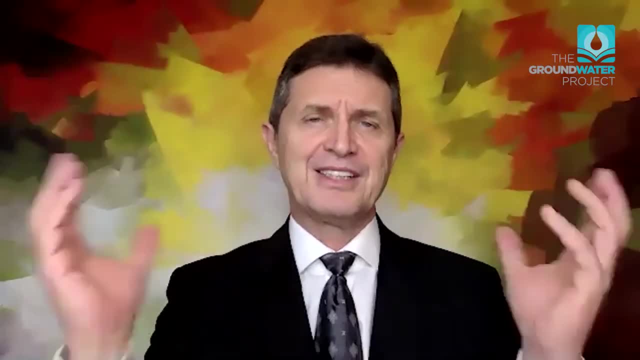 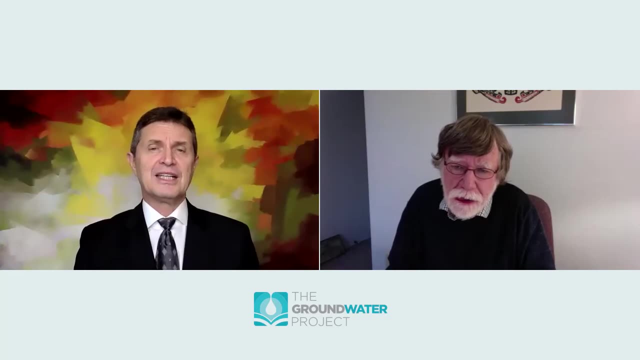 understanding, because we have the characterization of the, the, you know the mine itself, the whole thing, the project, and then you start the operations of the mine, When you start working in groundwater at that point, and how does it develop during the operations? What is necessary? Well, my experience is that 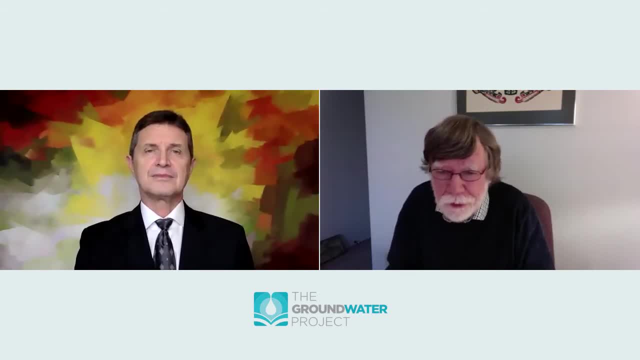 there's as much, if not more, effort put into trying to understand the groundwater system before you develop the mine, because it's part of the mineral economics. How much money do you have to spend to manage the mine environment? And then usually, once you're into operations? 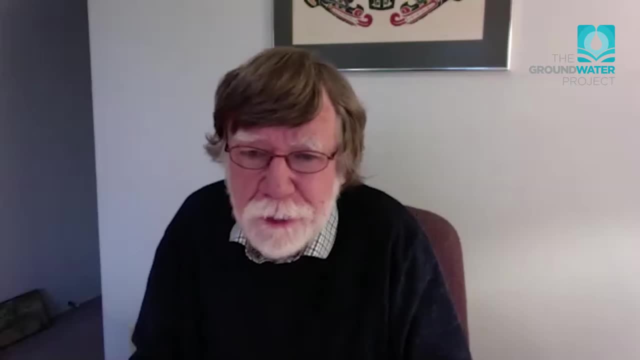 it's things might not have quite evolved the way you had anticipated, and so you do investigations to try and figure out: why are we having more inflow in this area than another area? So you have to mount another site investigation program. there It's often the case that 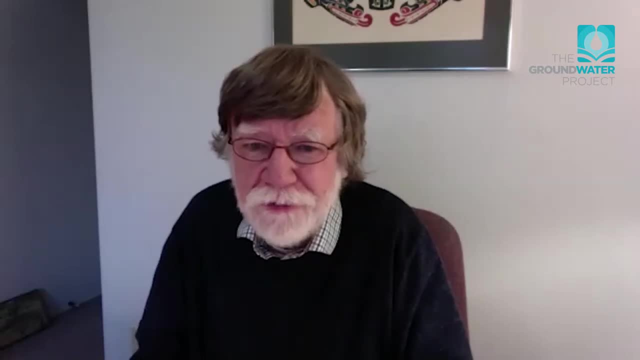 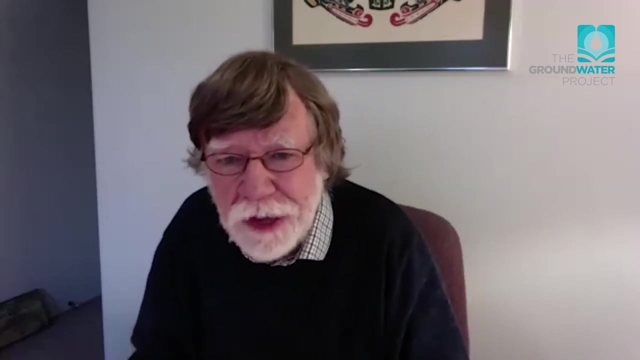 mines are developed in stages, so that you might have an initial phase one, do the exploration for hydrologic setting for phase one, and then, if the mine is economic, they might have an expanded phase, find more ore, and so there's another round of site investigation. that goes on with. 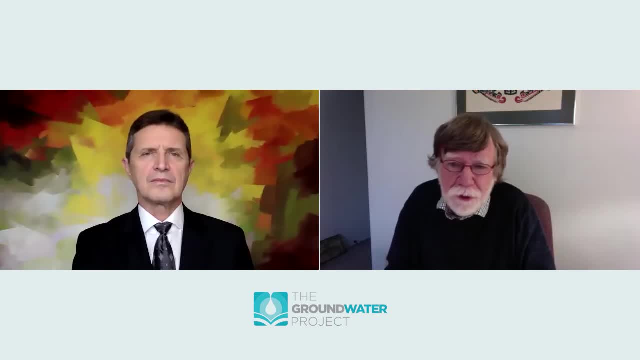 that activity. And then there's just the general monitoring of pore pressures around the open pit, monitoring of pore pressures and solute concentrations in the regions around a tailings facility or a waste drop facility to make sure that you're meeting requirements for environmental compliance. New site investigations and also monitoring. 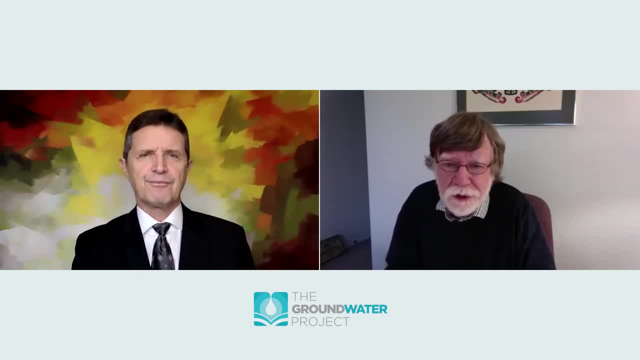 Monitoring is key to making sure that things are going as you anticipated. But you use the groundwater in the production as well. right, In preparing, separating the ore, right, That's right? Yeah, my earlier comment: the water's just as important, or almost as important. as the ore, because if you don't have the water, you can't process the ore right. You can't process it. That's the only company that has to do it. If you're using the water for a long run, you're only going to do it in the mine. but if you're using the water for a long run, it's probably not going to be sustainable, because if you don't have the water, you can't process the ore. 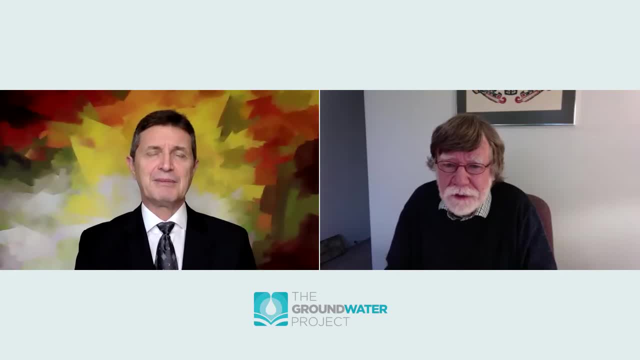 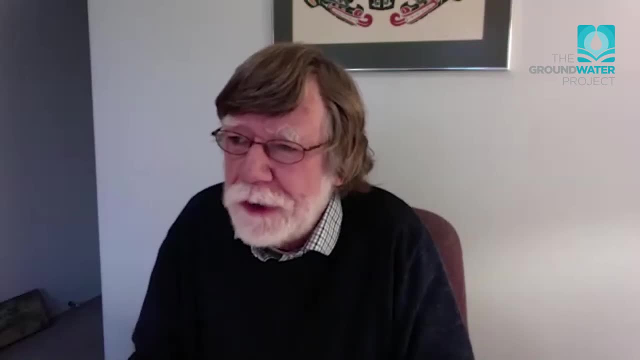 the ore, exactly, exactly, and so it's. it's not uh discussed much in the uh book. actually, i should mention this. there are are two topics that are obviously missing from the book, but just in terms of the scope in which i was set. one is the uh water supply development, uh for a, uh a mine site. 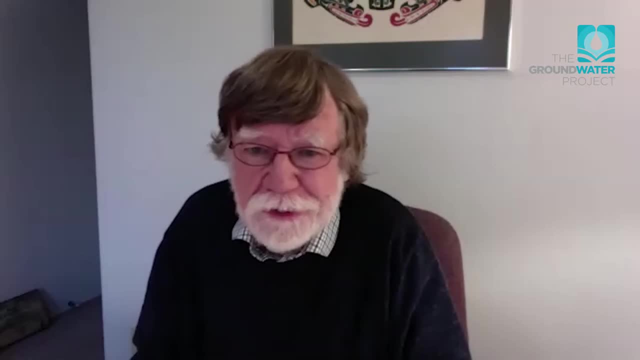 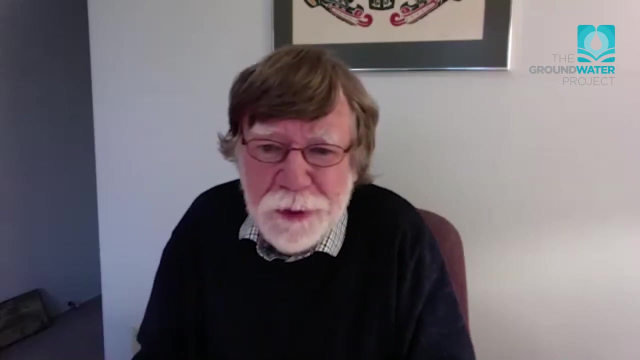 uh, that's aquifer hydraulics etc. so that's covered in other books. yes, and the other uh side that is not discussed is equally important to the physical side of mining and hydrogeology and that's the geochemistry which is acid rock drainage processes, and i'm assuming someone else will eventually be. 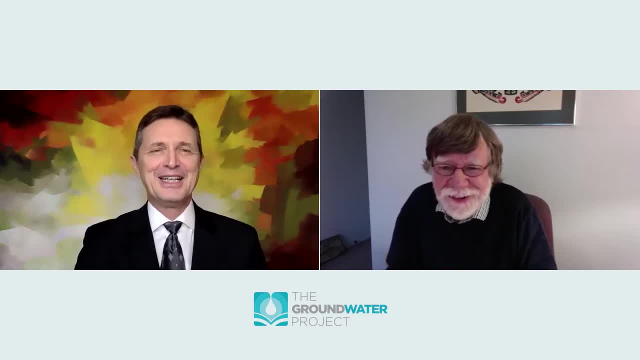 writing a topic on that. yes, we're working on that already. yes, but but you, you presented something you know for a hydraulic test there in your book with equation. that was quite interesting. can you talk about that? i put the equations in not very many of them because 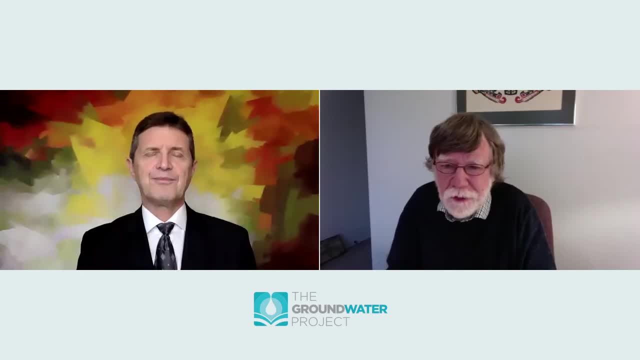 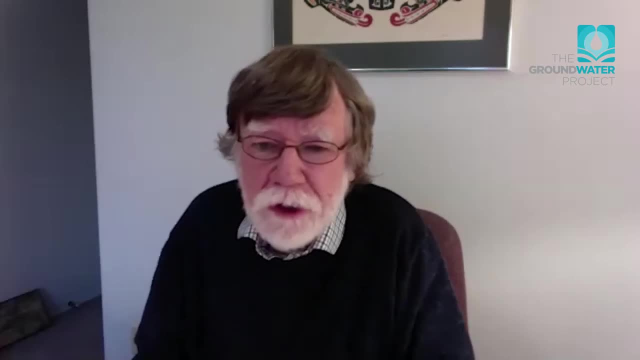 uh, uh of the- the message i was trying to get across, but principally in terms of illustrating concepts such as the equations we use to calculate solute loads to receiving water from a groundwater system, or the equation that, uh, you would use to predict when you might observe an impact of. 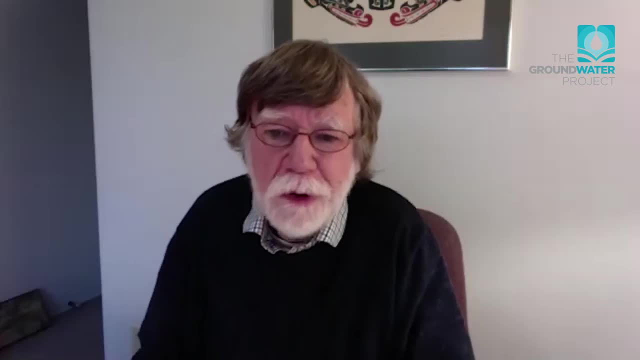 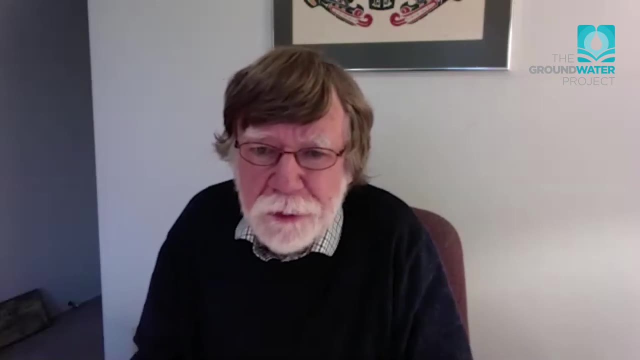 dewatering at an open pit mine on neighboring wells in the vicinity. so there are a few equations in the textbook. uh, there are also references to the equation that i was trying to get across, but this isn't a textbook. that would send you to other books that have much more extensive compilations. 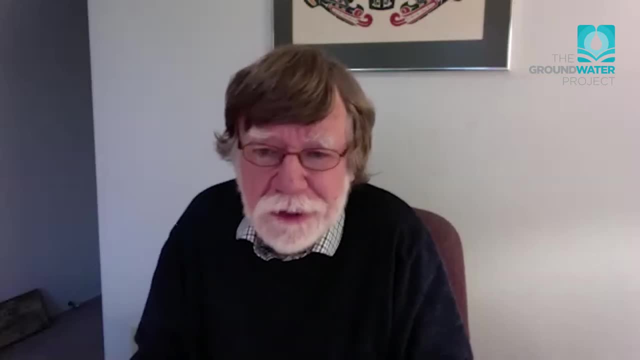 of equations used to predict uh, draw down due to excavations, draw down due to underground tunnels. but again, this wasn't a nomogram i was preparing, it was a textbook type material. so there's a few equations to, for pedagogic purposes, uh and the others are you find them in the references that? 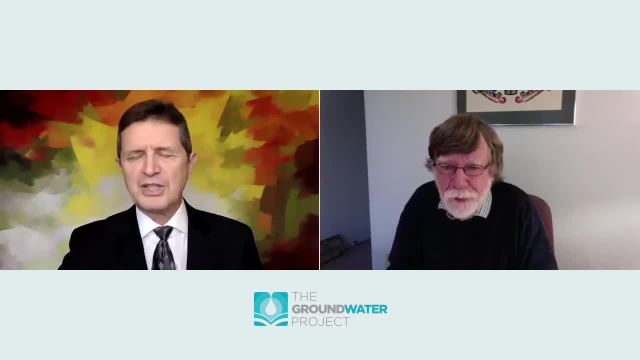 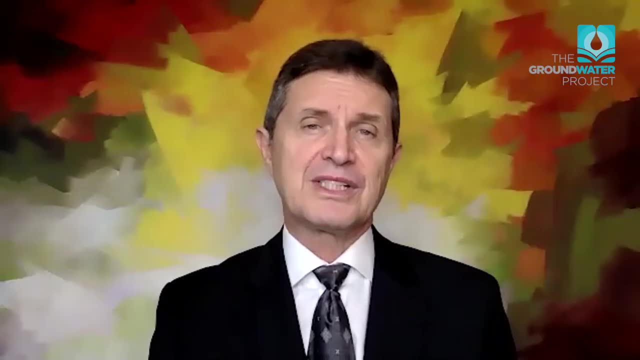 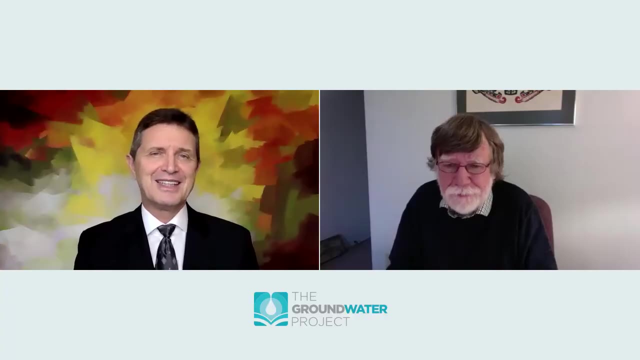 i incorporated in the book. yeah, no, i know because i've seen. i've been to one coal mine. you know, uh, in in in germany that was closed i don't know 50 years ago and you know the water table takes so long to recover. that, yes, but at basements and things, because people 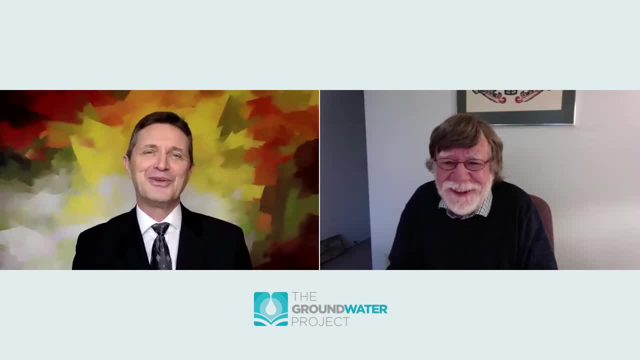 didn't even know. you know what was the original water table, uh, 200 years ago or something like that. but so there is the example that i i i mentioned briefly is that, uh, if you're mining water in an arid region, uh, it may take the water table centuries to recover. yeah, so you may also. 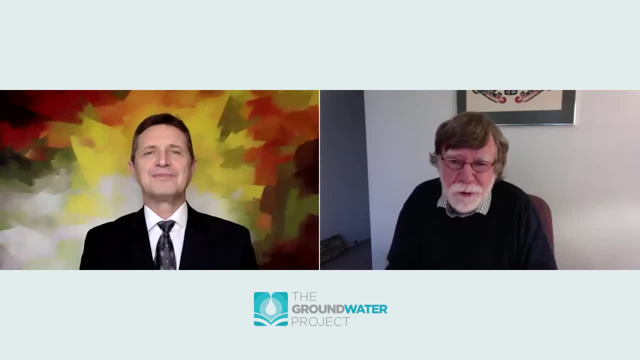 you may be thinking yourself as mining both ore and water. the water is renewable, but it's renewable on a time scale of centuries. the ore is not renewable, of course, unless there's a new intrusion coming in, but uh, uh, recoveries can take a long time. yes, yeah, this is quite important for. 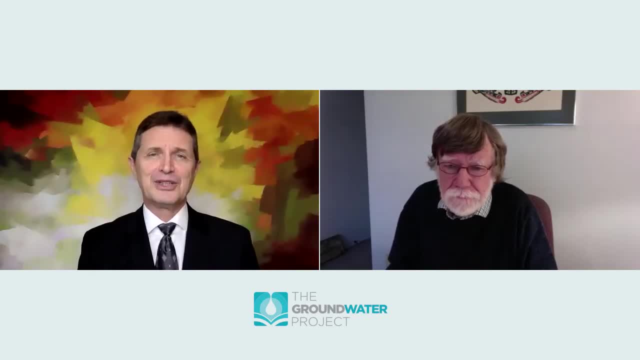 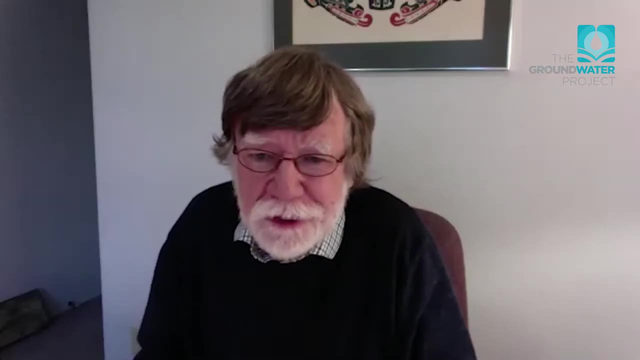 someone new in the field to know that we're talking about you know, a very long time, right? it's for you know, for some other generation to see the results after it's closed, right? yeah, and this same would apply to, uh, some tailings facilities, the tailings facilities. 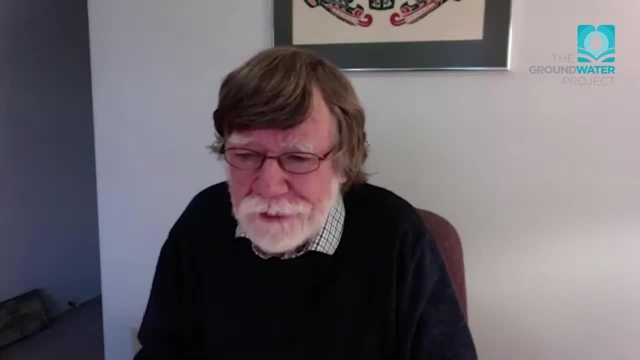 contain uh, the uh uh rock from which the? uh, the ground up rock from which the ore has been extracted, uh, usually deposited in a slurry, and it can take decades or more for the elevated water table in the tailings facility to recover the water table and the tailings facility to recover the. 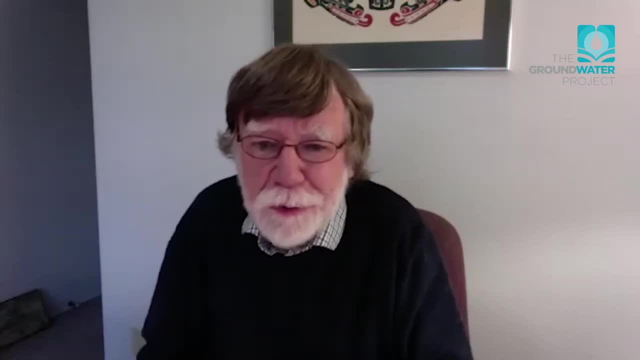 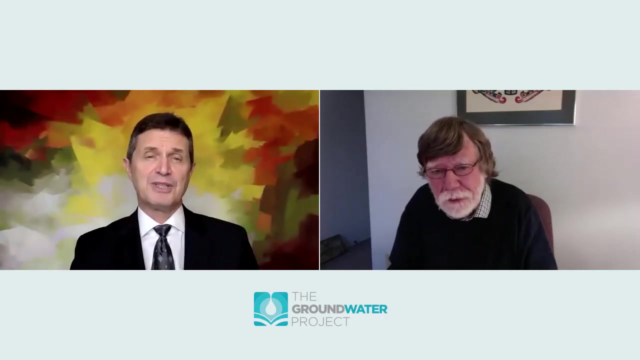 to drain down to, uh, uh, a new equilibrium condition, uh, in the closure landscape. so, uh, after mine closure, it can be decades or more. uh, that, uh, it could take for the tailings to drain. yes, well, that was my my next question, because you talked about, you talked about the tailings, you talked a lot. 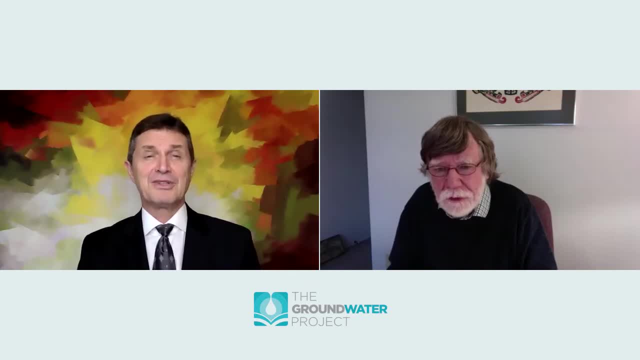 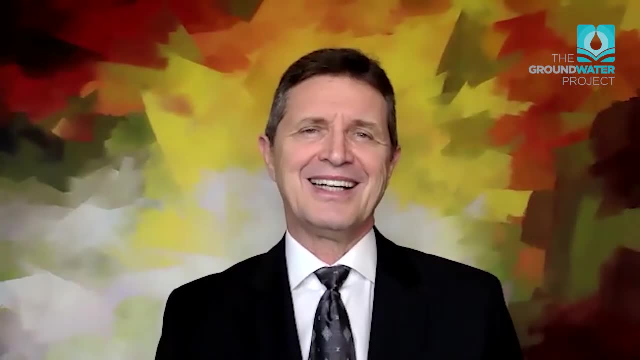 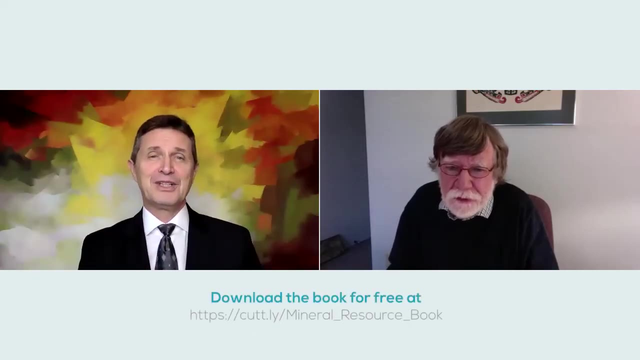 about tailings in your book was very interesting- some of the aspects because i worked with mine things, but usually as a remediation stone than i am. you arrive one when the the things is is already done, right, yeah, and your book you show how, how you build it and how water is important. can you tell us a little bit, uh, the? 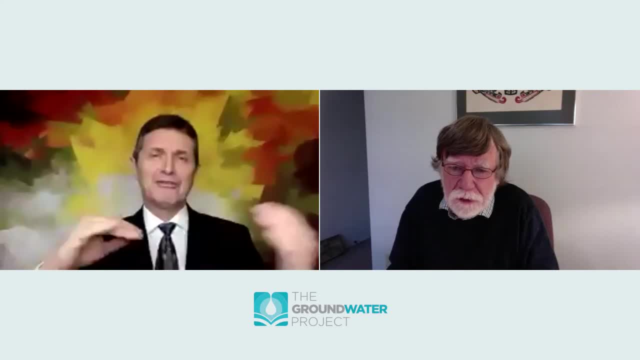 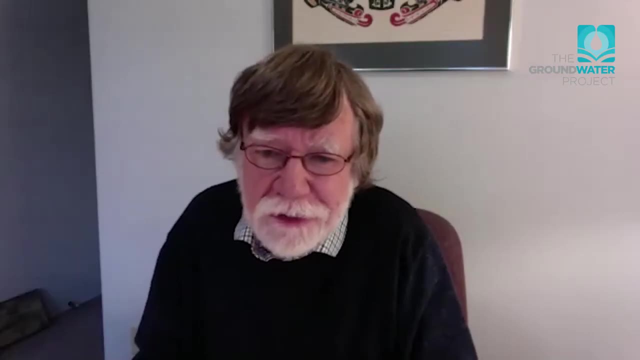 evolution of the of the tailings pawn and how you know the difference that we have, because you mentioned that on your book. could you briefly tell us about that? well, uh, tailings ponds, uh will invert, will will have a tailings dam, so they have to build a, a tailings dam. usually it's built in stages through the life of the mine, so it's raised every year, every two years, to meet the required storage. uh uh, that is needed by the production from the mill. so it's not like a hydroelectric dam which gets built in one stage. your damn tailings. 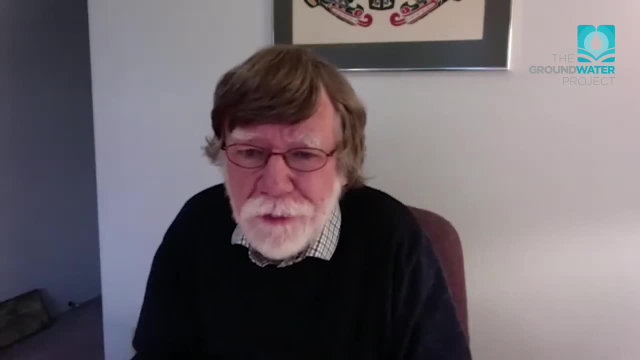 dams are raised up, in lifts occurring every year and, uh, you need to understand your volume of tailings that are produced, uh, the rate at which that's occurring and the rate of which it's going, at which you have to construct your dam, The rate at which you have constructed dam. 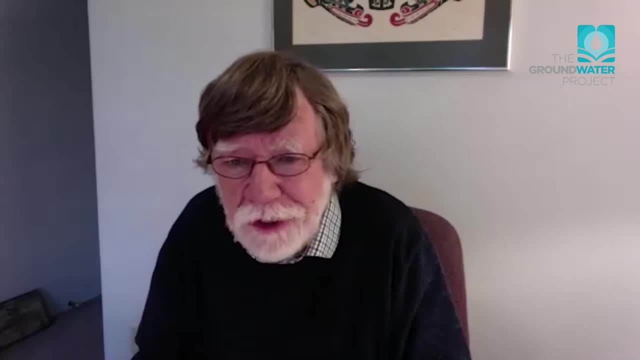 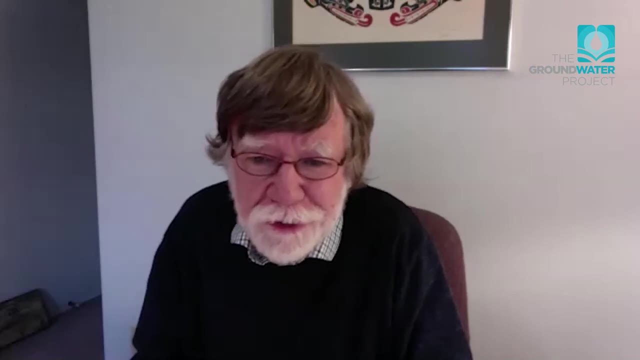 can be sometimes limited, because if you construct it more quickly, you'll generate higher pore pressures in the foundation, and higher pore pressures reduce the shear strength of the foundation materials, And so there's all kinds of issues you need to think about in dam construction for tailings facility. 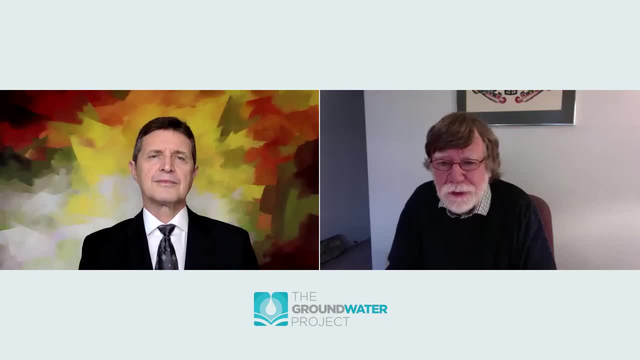 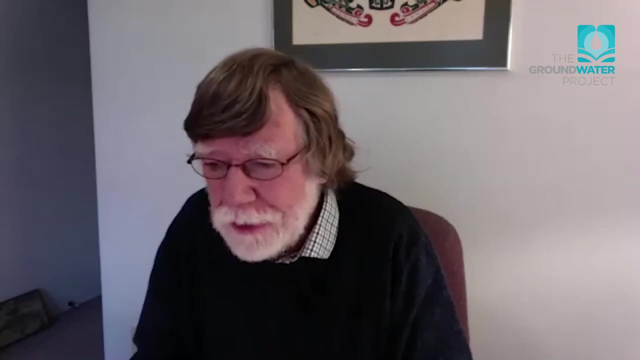 that link to the hydrologic system as well. That's one side of it, The other side of it. as water level rises in the tailings pond, there's an outward hydraulic gradient seepage to the surrounding environment, So the facilities have to be designed in a way. 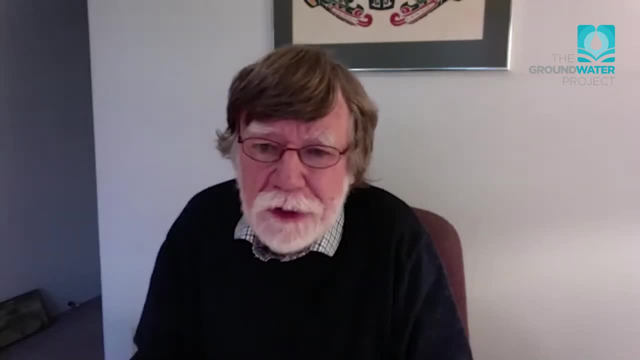 that keeps the seepage rates at a level that meets the attenuation capacity in the surrounding streams or is in compliance with regulatory limits on solid concentrations in nearby monitoring wells or compliance wells set by the regulatory authorities. It's very nice. So you talk just to illustrate. 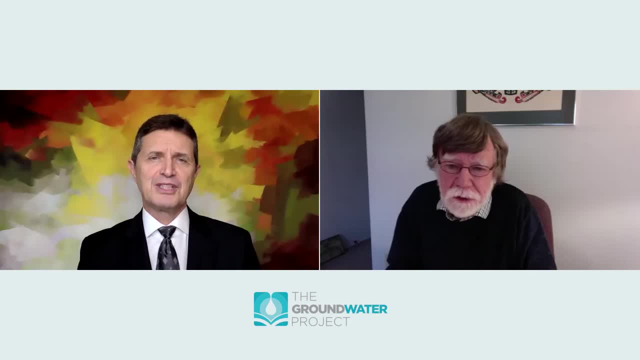 you talk about the beaches, the size of the beaches that are produced. How are the beaches produces? Because when someone think about a beach, they're thinking about palm trees and things like It's just the same, but no palm trees. So you have the. typically, there are two ways of doing it. 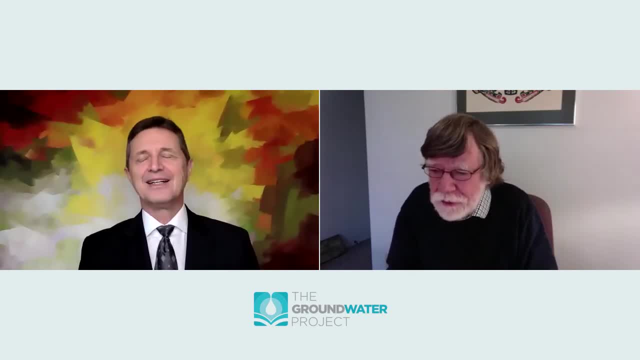 but the one I'll speak to here is they might be discharging a tailings from the crest of the dam and the water pool forms away from the dam, which is a safer configuration, And as you discharge the tailings, tailings have a broad range in grain size usually. 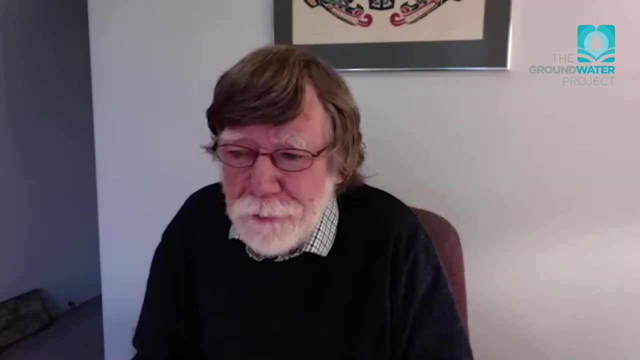 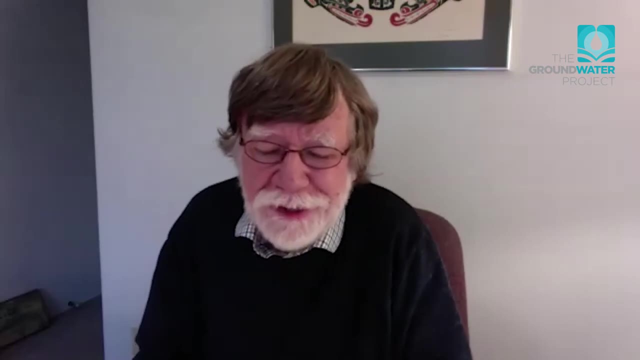 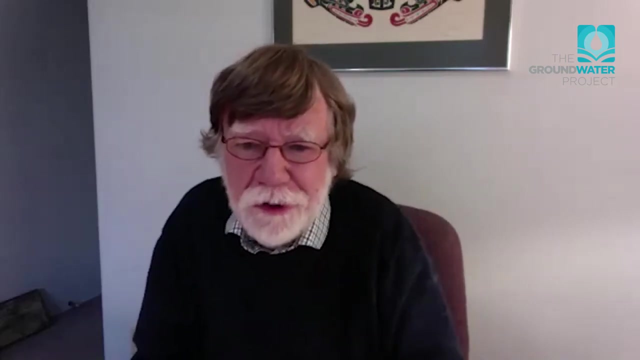 not always but usually they do And there'll be a medium grain sand to silt and clay-size particles. So if you deposit that into an open area, the medium grain sands are gonna drop out first. I know finer grain material will be carried further away into the water pool and just over time that 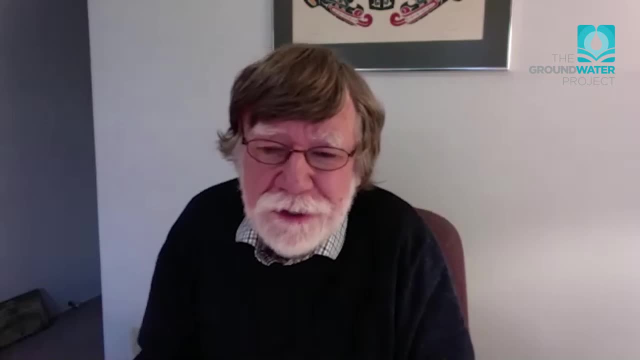 naturally builds up a sandy beach in front of the tailings dam. so it's a, it's an element of good practice to actually get a beach developed so you have the pool, water pool, away from the dam, away from the dam. yeah, so that's, that's the advantage of a tailings beach and we talk about. 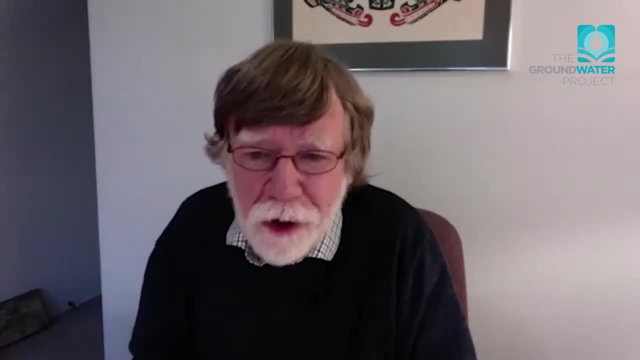 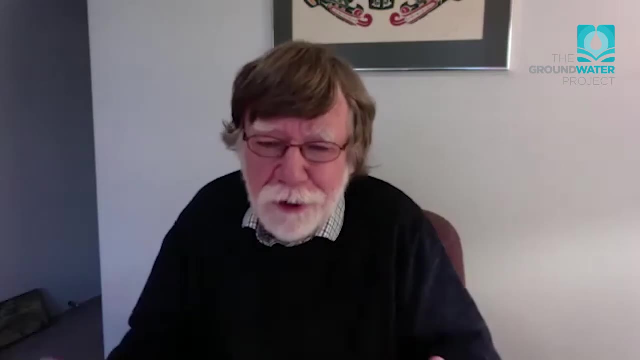 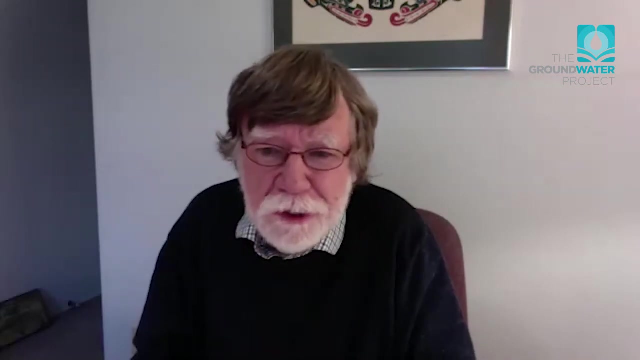 they talk about tailings beaches above water, tailings beaches that develop below water, but it's just the distribution of tailings within the facility and the hydrological aspects of that is. if you're looking at a tailing facility and saying where does the leakage most likely to occur, or 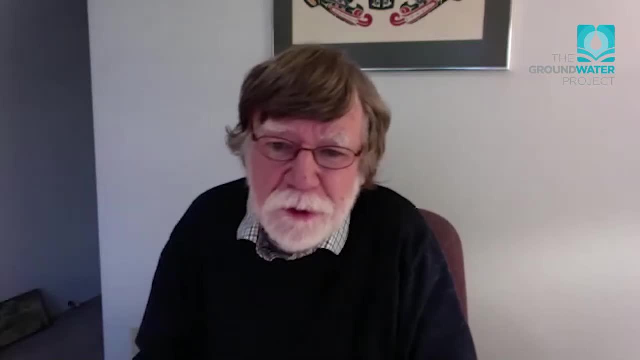 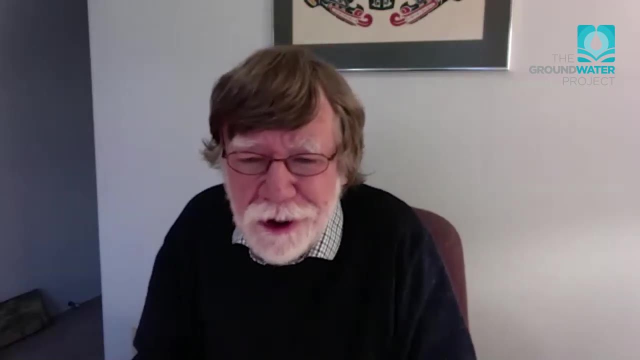 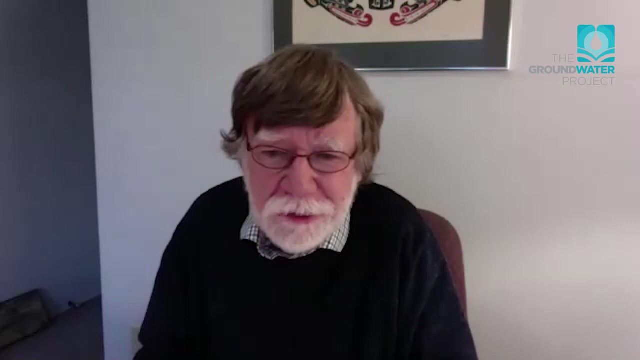 release to the surrounding environment. it's going to be where the tailings are most permeable, because tailings permeability determines leakage rates, and so most of the leakage will be concentrated in the more permeable tailings, and much lower rates of leakage would be occurring in the finer tailings. 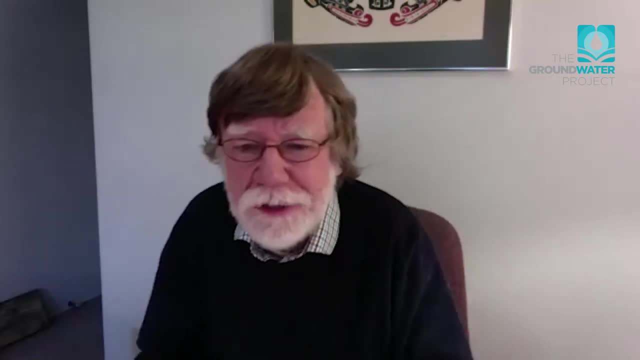 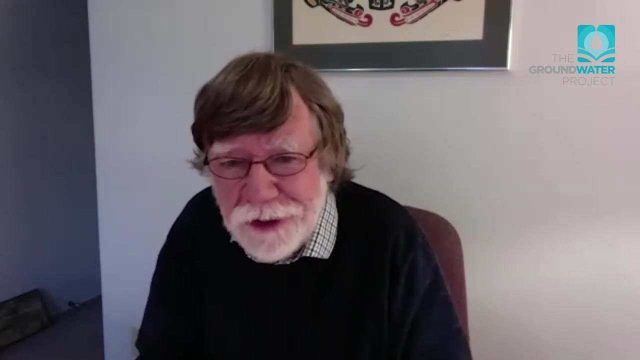 which we call slimes, so that structure inside a tailings facility is. we sometimes build that into the hydrogeologic models that people use to assess seepage pathways, seepage rates, so they impose a stratigraphy, if you like, for the tailings deposit, just like we have to analyze the 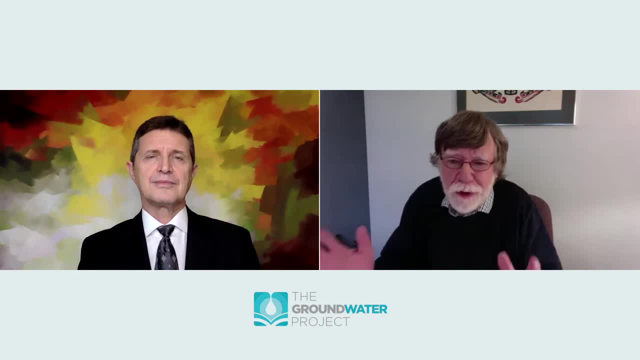 stratigraphy in a in a water supply problem for a you're you're in that water supply problem for a deployment problem, or what maintenance advisors advise you? average for more detail on what sort of drainage needed to be done and so on. so basically, how some things evolve aroundığ are left. 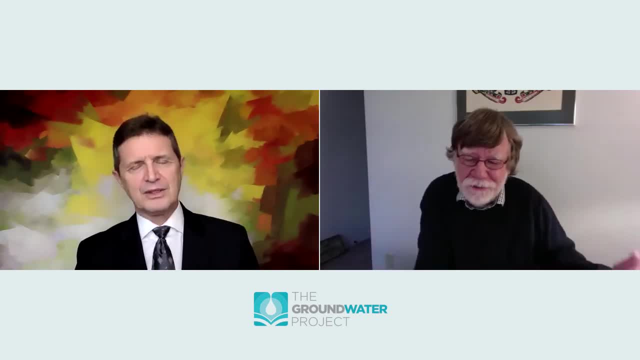 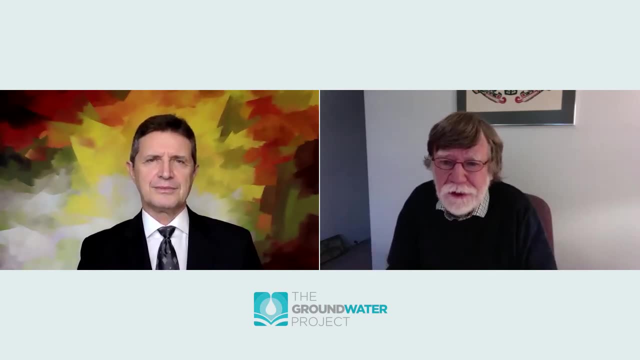 and we eliminate the most predominant��분 that still happenne and we eliminate the most predominant affiliates that still have knowledge and there are like whether the main air lookoutżej will have the knowledge and control to do. it'll be a lag validation or something like வ. 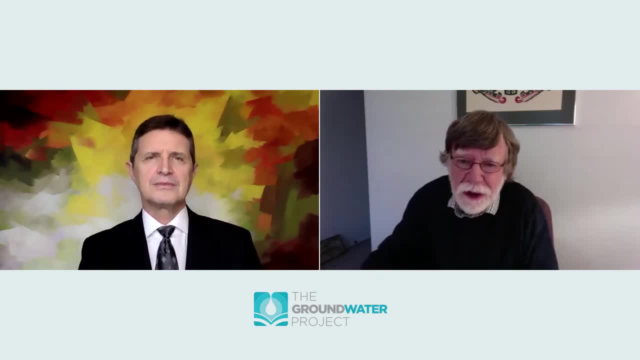 portion of material settled out. They moved the discharge locations around the dam, So it's not the same position every week, every month, And that leads to a quite a heterogeneous system of tailings. Okay, but just a curiosity, you use that. you have that as a record of how it was built. 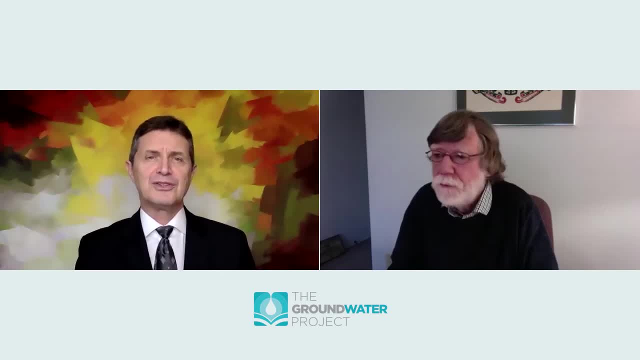 or you have to drill to study the heterogeneities within the tailings. You might know the general patterns, as I just described, but if you need the detail, you would have to drill to get that information. Drill, or there's another technology. 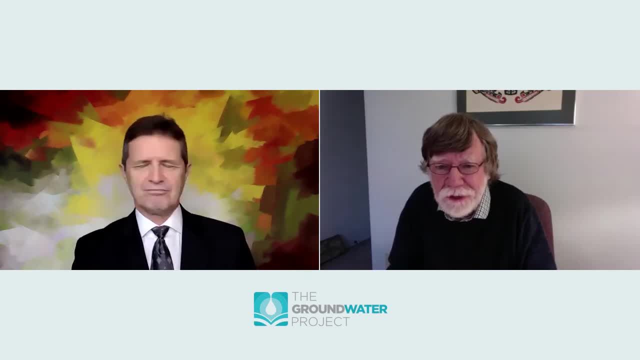 which cone penetrometers, CPT testing, So you can go out onto the tailings beach or on a barge and push a CPT probe and you can characterize the lithology that way. Okay, okay, that's okay. So, but then it's usually. 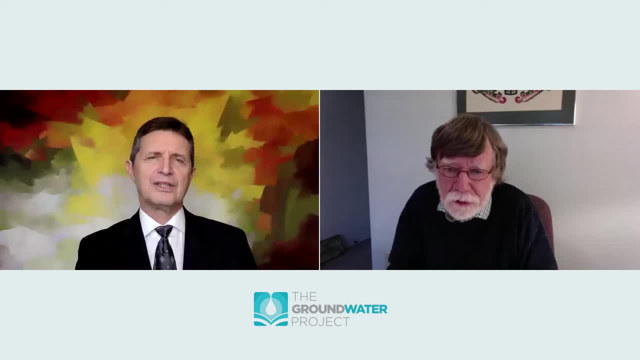 it's saturated. So cone penetrometer that will do the job. I think right. Yeah, tailings usually have a during the operating phase. If you go to a small tailings facility in an arid area 10,, 20 years after mining is complete. 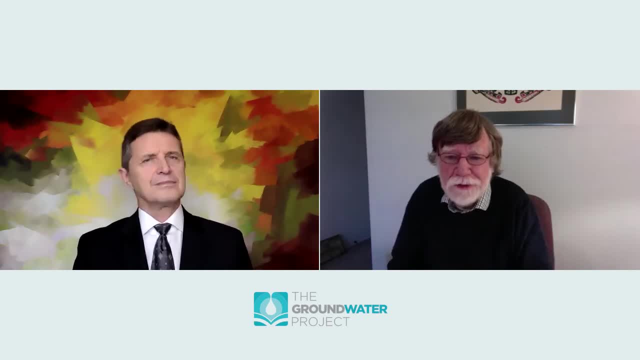 it'll be a stack of sand, The water table will be low, the base of the foundation. So that's a possible closure configuration. Okay, In the long run, how does the plume develops and how does the mining companies deal with that? 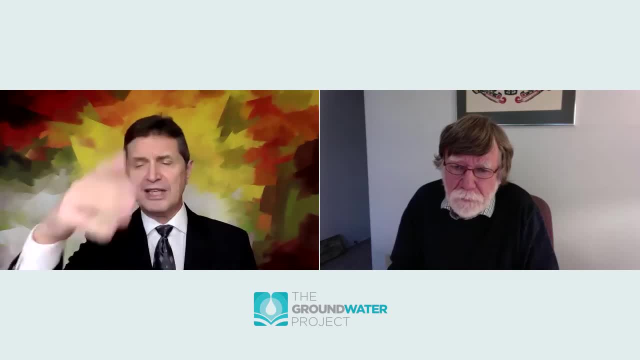 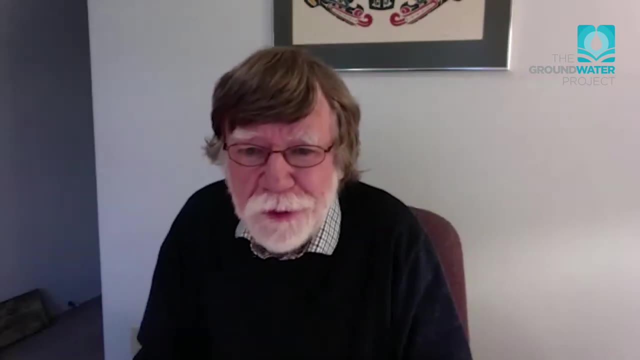 Do they have to take care, monitor the plume development, intercept it? How is it done? It depends on the jurisdiction you're in and what the mining company agreed to at the time they received their permit from the government to develop the plume. It depends on the resource that developed the mine. Some mines have made the commitment to have a de minimis release to the environment, which means as small as practical. you can't make it necessarily zero, So a de minimis release to the environment. 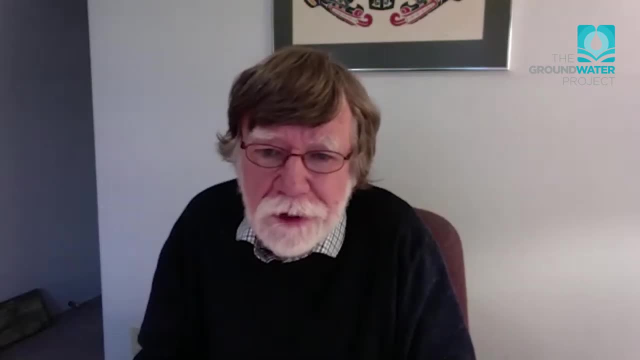 And to do that they often use a pump back wells. So, just like at a contaminated site where you have a pump and treat system, you can imagine having a pump and treat without the treat, because usually it's pump and pump back and then pump back. 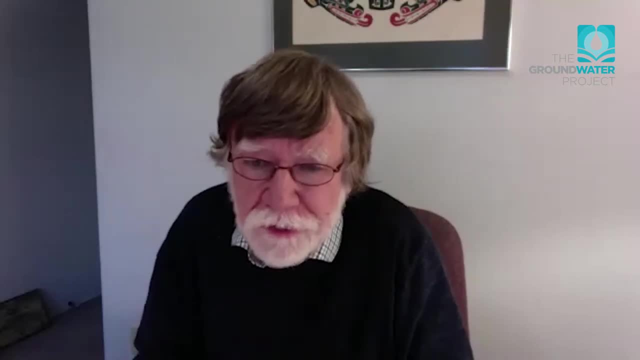 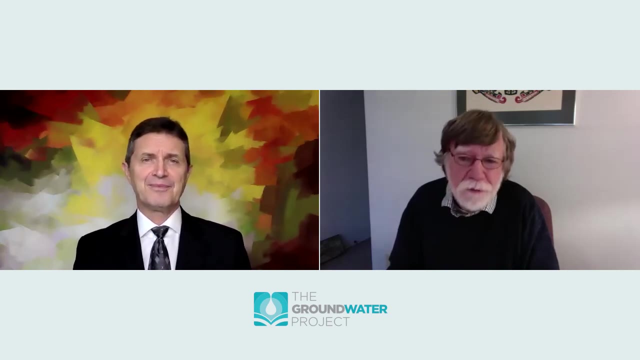 You can imagine having that pump back and pump back into the tailings pond during operations. Enclosure- Is this water usually used in the process? Maybe That water's then reused in the process? So yeah, it is reused in the process. 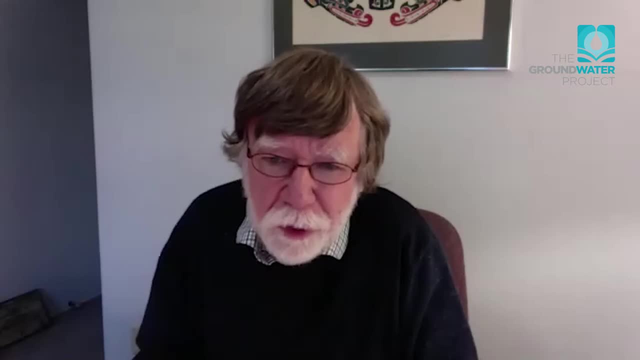 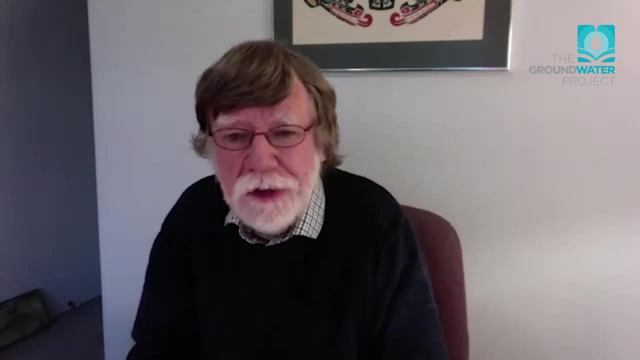 Enclosure when they're no longer using the water. in the process, you might have a pump and treat system, So enclosure- you might be pumping the water that's leaking out of the tailings facility, out of the ground to a water treatment plant. 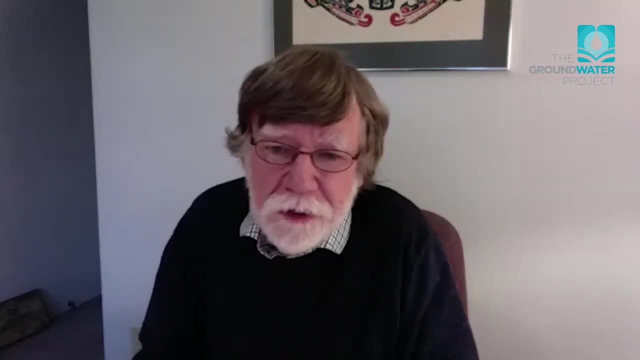 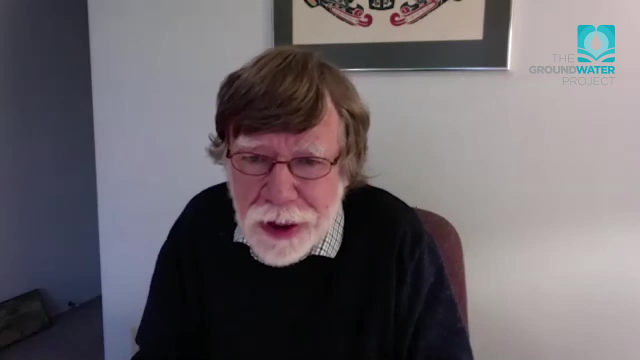 where it meets the standards for release in other just jurisdictions. you may have a a certain solute concentration limit that you're allowed to have for selenium, for example, or or sulfate, and in that case you might be able to manage your environmental obligations through using various low permeability cutoffs. 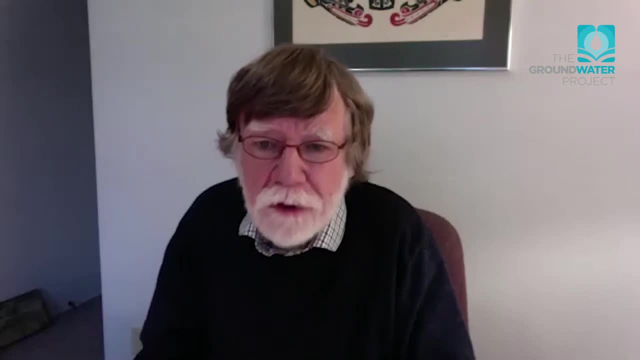 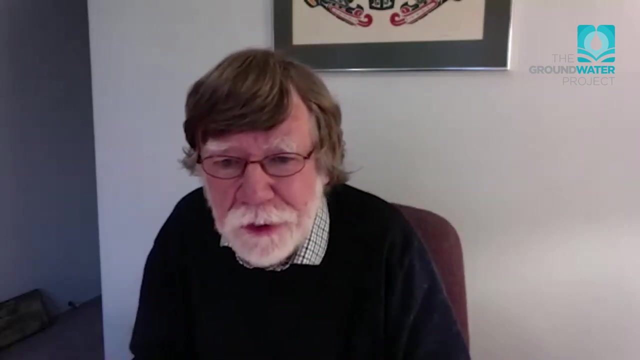 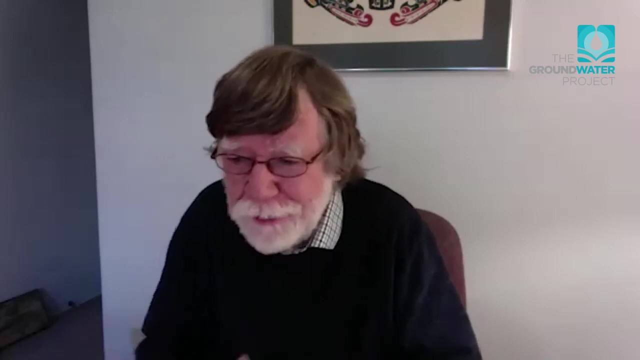 uh, barrier walls, slurry cutoff walls. so those are all different kinds of strategy. much like thinking about how do you control contamination at a contaminated site? yeah, those same concepts carry over to how do you ensure long-term protection in the environment? uh, at a around a waste rock facility? uh, a mine site? we've talked about your background at the. 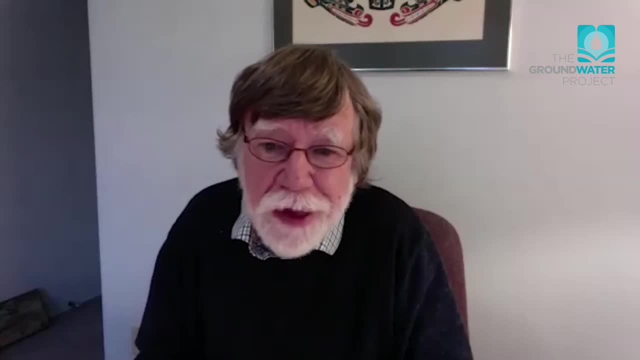 university of walu. they have a long history there of using reactive barriers. uh. reactive barriers are used at mine sites. uh, there's there's some here in canada. i'm familiar with uh in other countries as well, so the whole range of tools we use for contaminated site. 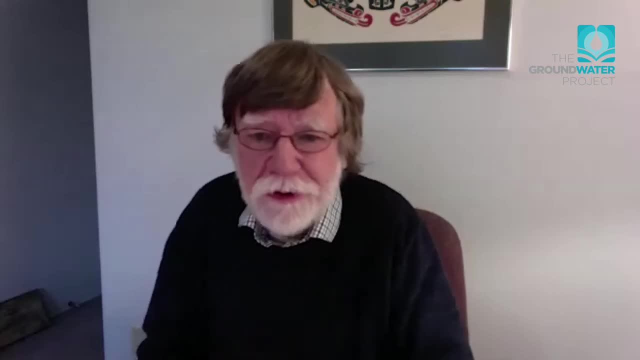 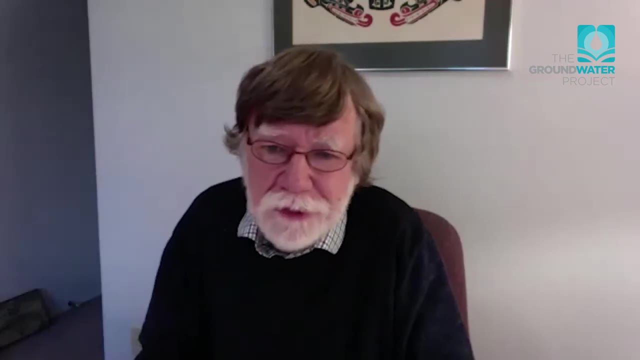 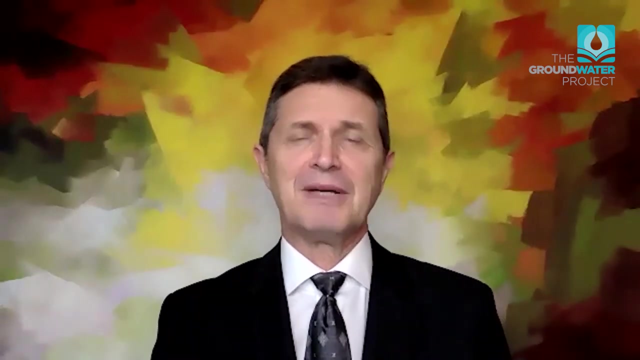 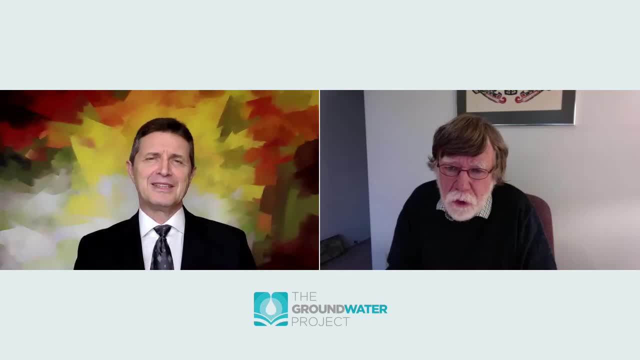 around the pillar. you know the, the contamination and different components that we, the plastics, were present. we we didn't actually have to prepare the uh materials for ourorp nicely, and so we haven't really took the practical sort of steps that are putting us in the right direction. and you know we will be able to work with a number of types of projects, like thank you or government or many other things like that that the other problems do play a big bottle of. so you already have phase one, but- and look at the businage problem- so i've gone to plant a little bit. 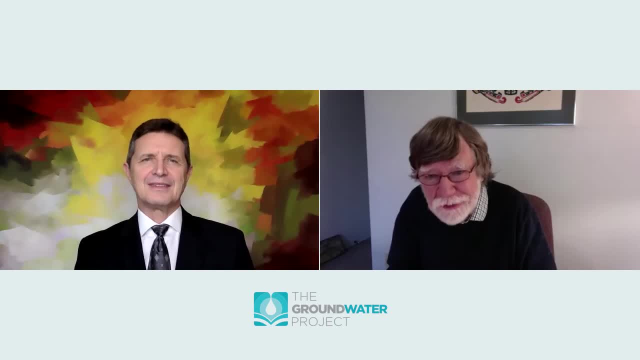 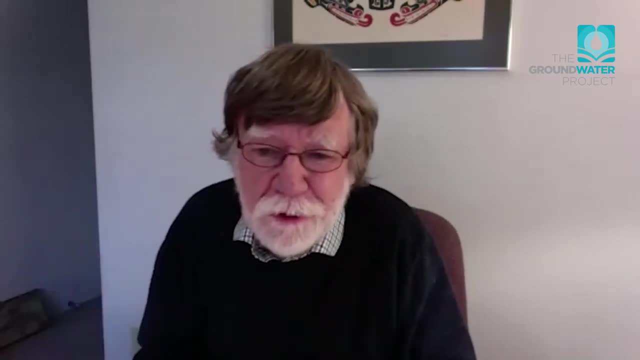 that's when reactive barriers make sense, okay, whereas if you're going to be at a closed site where they know it's, for various reasons, going to take a hundred years to close the facility, or that's the period of time that they're working to then a water treatment plant, because you'll 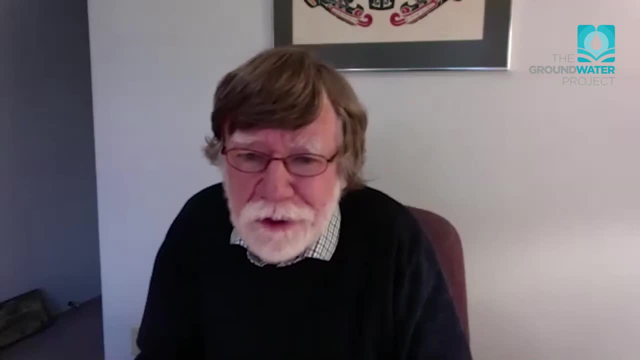 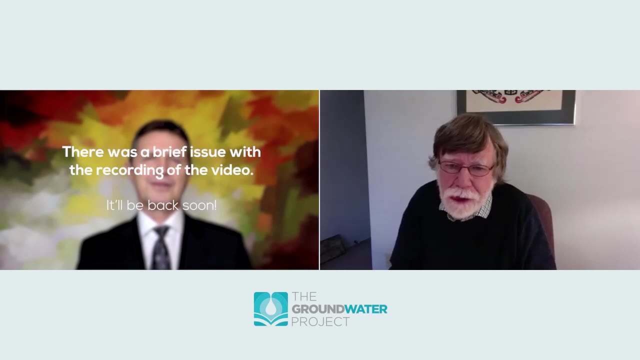 have people working there, you'll have power there, etc. so, again, local conditions determine your strategy for for for plume management. yeah, okay. so uh, the when you talk about the mine closure, well, how important is the groundwater? because people think most of the times when you talk. 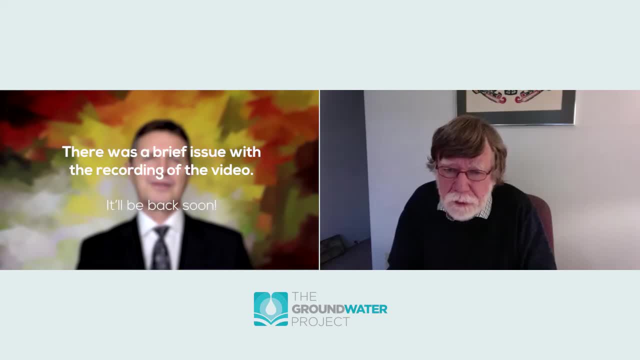 about my enclosure. i, i, i worked on a site here in brazil that was closed in uh, 1968, right, uh, i was born. unfortunately, i was already born by that time and you know, uh, the public attorney went back there because they were worried about you know. 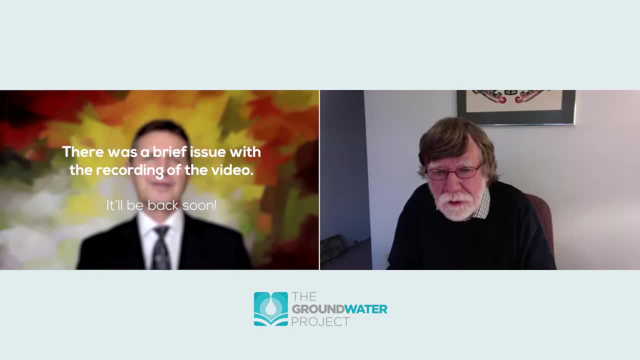 the, Actually the degradation of the area. actually, visually, the impact is way more important than groundwater, because people still don't see groundwater, right? Yeah, But we still have a long way with the groundwater contaminated site. If you don't care, you just leave it there. 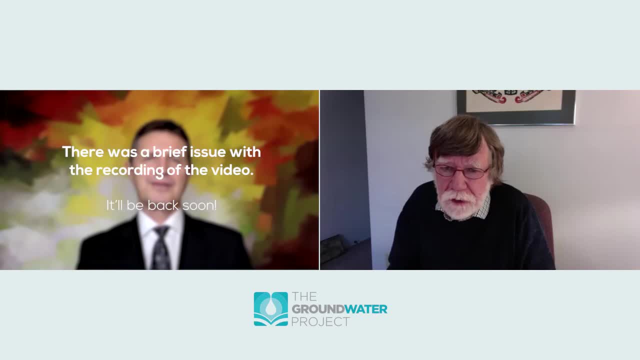 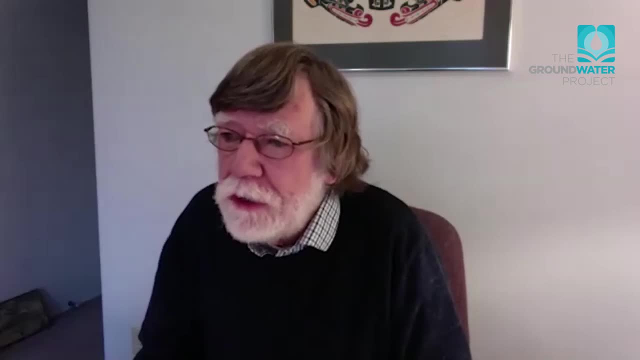 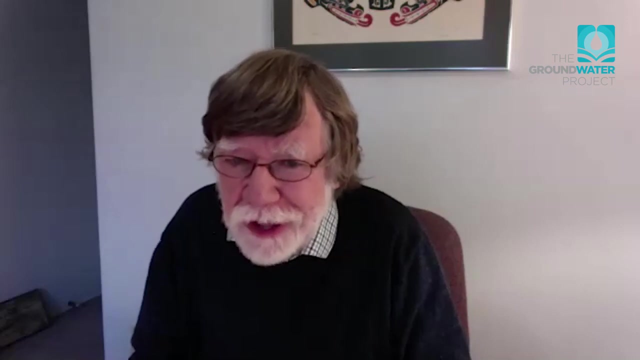 So how important is taking care of water after the mine closure? From a groundwater perspective, the real issue is focusing on after closure: what will be the groundwater recharge rate through the tailings facility or through the waste rock facility, And what solids will be picked up as that water is infiltrating through the tailings or the waste rock. 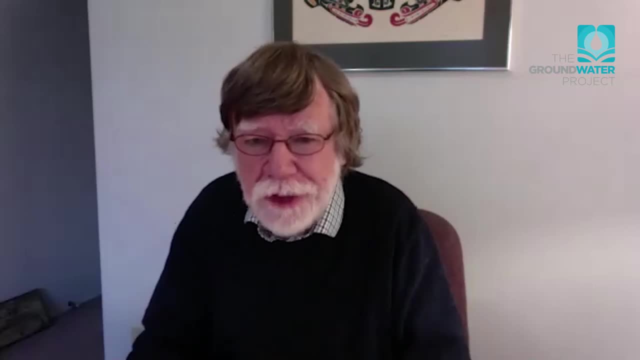 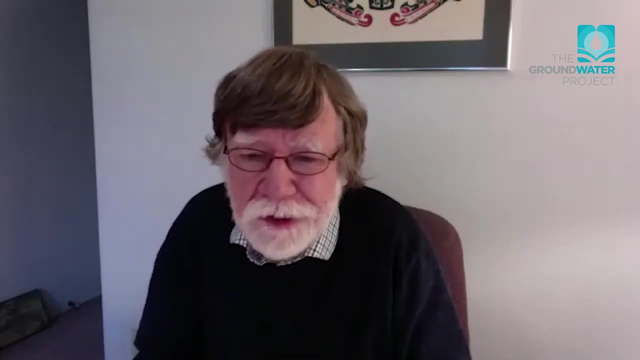 Usually in closure. it's going to be Partly through the unsaturated zone, then the saturated zone. So that's where this hybrid geochemistry topic comes into play, Equally important for assessing what the impacts would be as the flow itself. 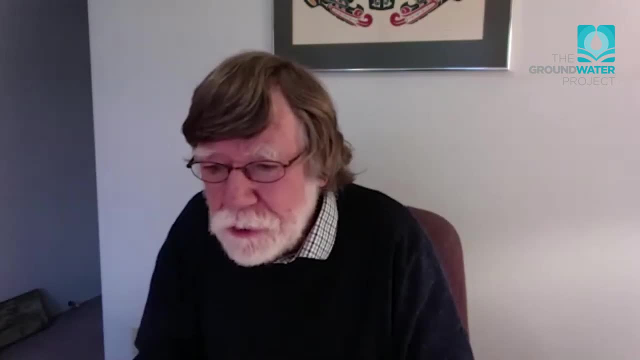 But ultimately what you're trying to do again in closure is to reduce the loadings to an acceptable level to meet environmental standards, And that usually would imply in more humid areas where you have water surplus, you're going to have some kind of water cover or lower permeability water cover. 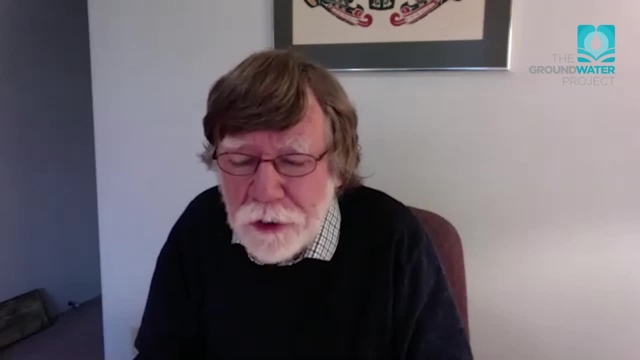 You'll have diversion ditches because you want to reduce the amount of water that infiltrates through the top surface of the mine- waste, whether it be tailings or waste rock- So it's really an infiltration control. There are other aspects, of course, as well. 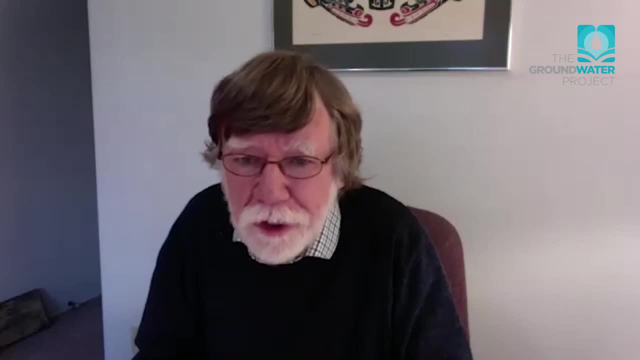 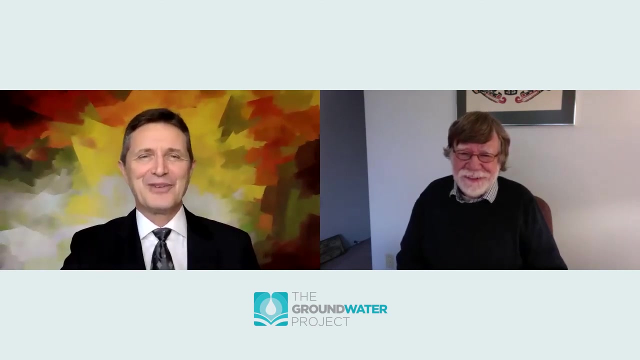 But from a groundwater perspective, it's how to reduce the loadings to the receiving environment in the closure landscape, which is reducing infiltration. Okay, Les, that was very nice talking to you And I really enjoyed your book I recommend to the readers. could you please make your final considerations for people who wants to read the book, people who wants to take their career in that area, please? 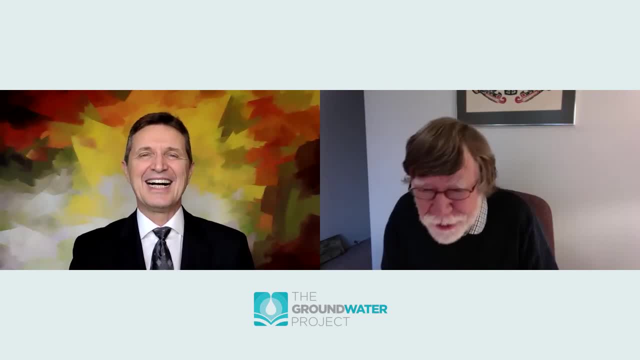 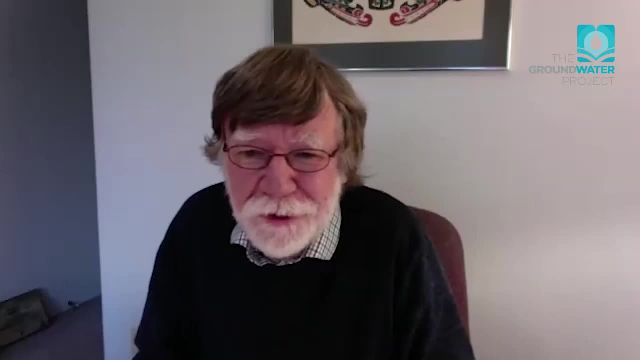 Well, I hope you enjoyed reading the book as an introduction to the field And if you get enthused on it again, there's some references there that take you to the literature for a deeper dive into the topics And as a career. water and mining. 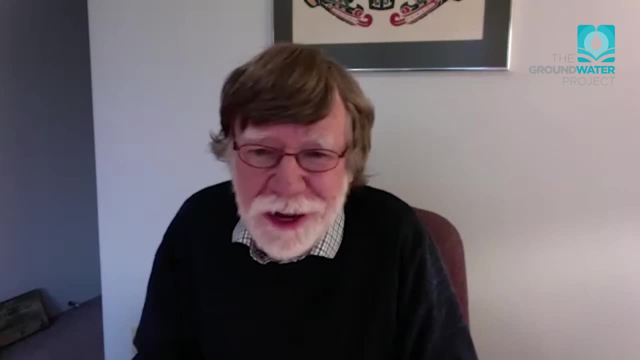 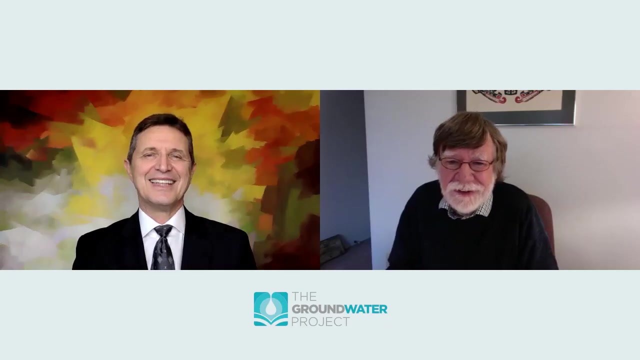 Mining. Mining's got a long path ahead of itself as a viable industry, And so you can imagine having a full career in working in mining and hydrogeology. They're good opportunities, All right. Thank you very much. I enjoyed your book.